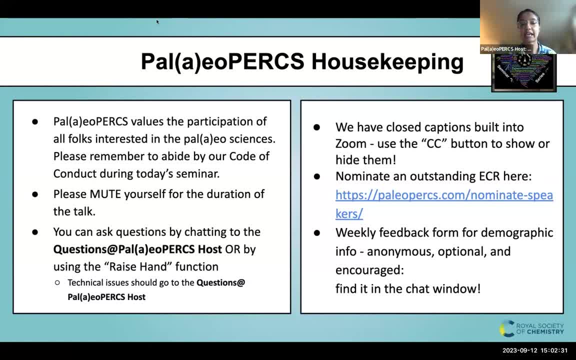 going to be Elizabeth, Or you can use the raise hand function at the end of the seminar. We will unmute you and you can directly ask Russell your question. Any technical issues that you faced during the seminar should also go to the questions at Pandioporex's post. We do have Zoom captions. 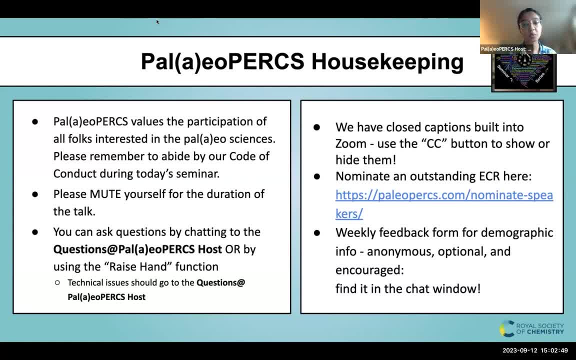 so you can use the CC button to show or hide them. You will find two links in the Zoom chat. One of them is for nominating an early career researcher to give a talk at Pandioporex and the other one is an anonymous, optional and highly encouraged weekly feedback form. You will find both of them. 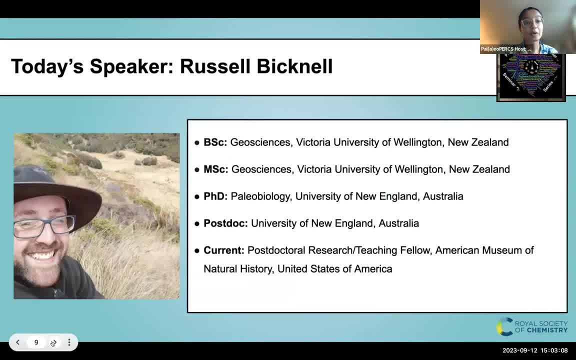 in the chat With that. we are very excited to have Russell. He did his bachelor's and master's at the Victoria University of Wellington in New Zealand, both of them in geosciences, followed by a paleobiology PhD At the University of New England in Australia. he also did their postdoc there. He is currently 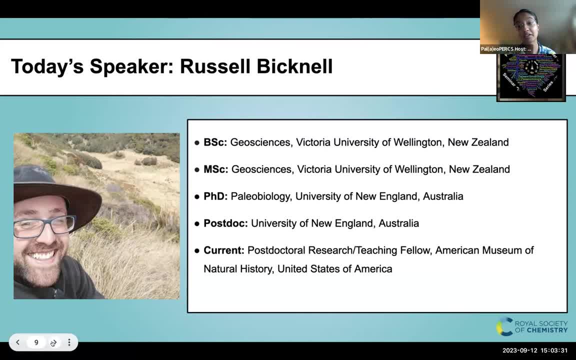 a postdoctoral research and teaching fellow at the American Museum of Natural History. With that, Russell, feel free to take over the Zoom screen share and tell us all about trilobites. Okay, thank you very much, Let's get this going, Okay. hopefully everyone can see that. 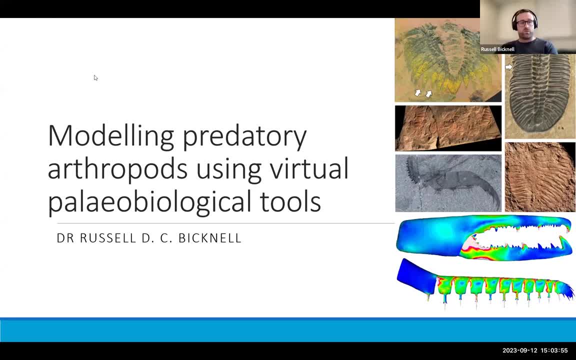 So, yes, thank you all for, I suppose, coming to the Zoom today, It's my pleasure to talk to you all about some of the fun and funky research that I've been doing over the last seven years, in which I've tried to use an array of three-dimensional tools to kind of tackle questions. 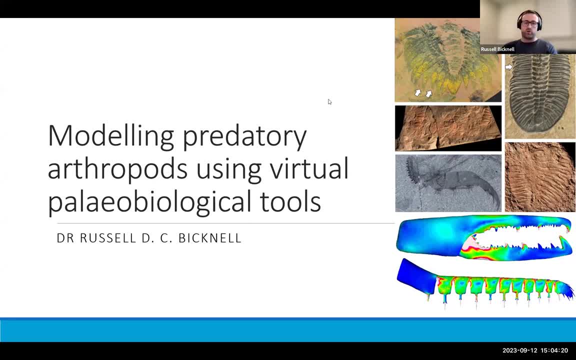 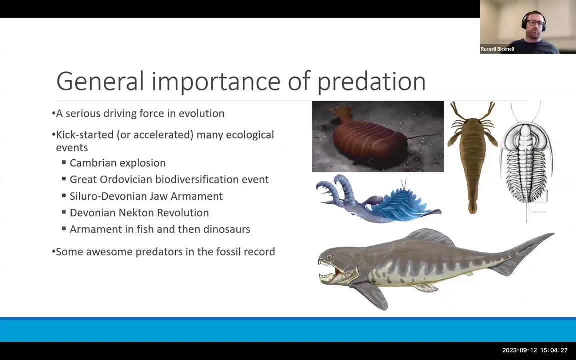 within arthropod paleobiology to understand things like predator groups. So why do we care about predation? Well, predation is generally thought to be a pretty serious driver in terms of evolution and the rise of different predator groups has thought to have either kick-started or really accelerated an array of ecological 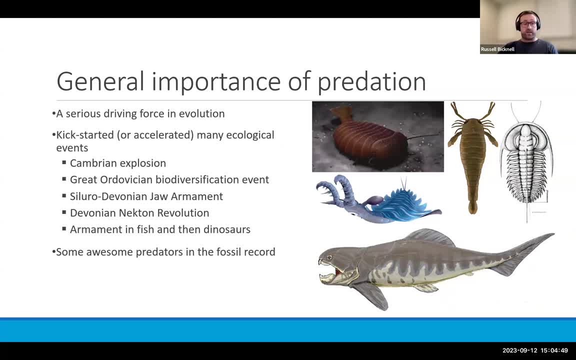 events over deep time. This includes things like the Cambrian explosion, the Great Audubition Biodiversification event, the Siluro-Devonian jaw armament, as well as the rise of planktonic animals within the Devonian, and then the armament of fish. 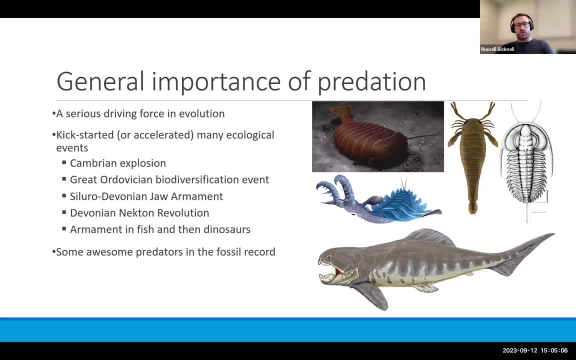 and then, of course, into more recent Mesozoic dinosaurs. Beyond that, though, predators are pretty awesome, and we can look at an array of their morphologies that we see in the fossil record to understand how they've been so successful. So how do we look? 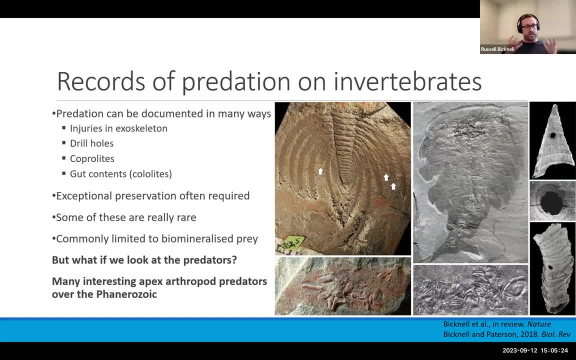 at them within invertebrates in general. Well, we can look at injuries in exoskeletons. So this is a trilobite here that's got some spines that are no longer there. That may have been a molting complication or it may have been predation. We can look at drill holes. We've 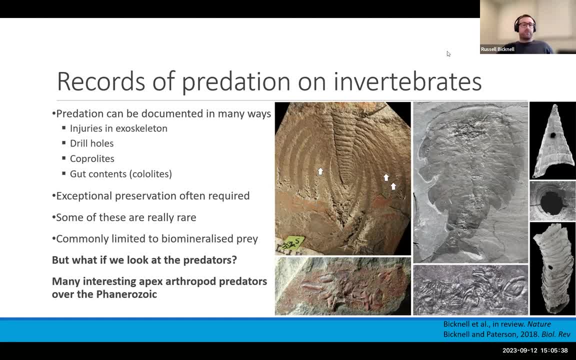 got a couple of examples over there, drilled shelly things. We look at coprolites, so the remains of fossil poop. An example down there from the Emu Bay Shale in Australia which has some trilobite fragments in it And we can look at the. 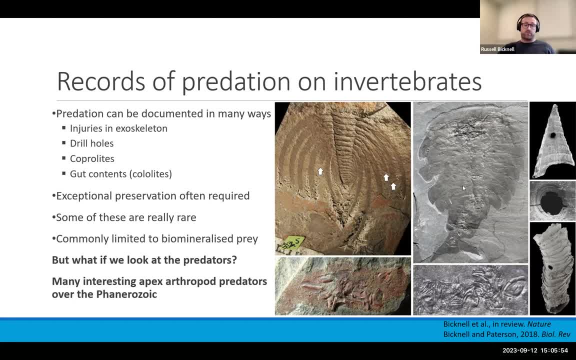 gut contents. So this is a really exceptional specimen of Sydney, an expectance from the Burgess Shale. So this is a close-up of what's in this animal's guts, showing us that this animal was eating some kind of shelly organisms. Usually we need exceptional preservation to 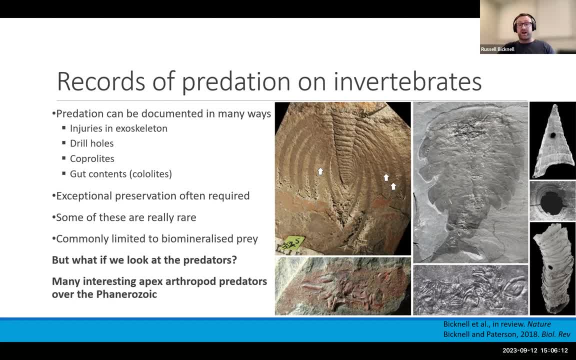 observe these sorts of interactions And really almost ironically, the more informative the specimen is, the rarer it is. So I think there's like maybe five specimens of Sydney in the Burgess Shale, which is of course beautifully preserved- that has these sorts. 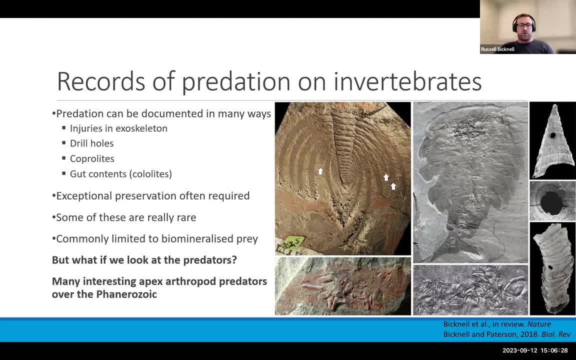 of information And it's kind of annoying. So we're often limited to looking at biomineralized prey and the results are either failed predation or successful drilling predation. But what if we change the narrative? What if we look at predators as opposed to the prey? 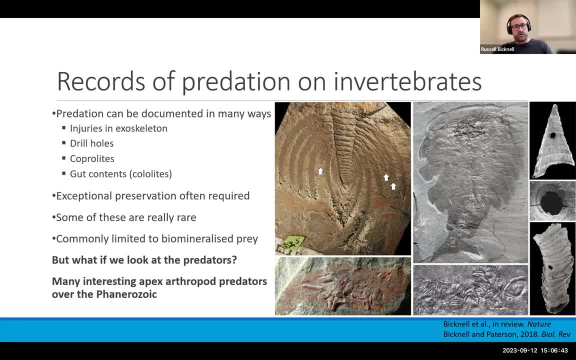 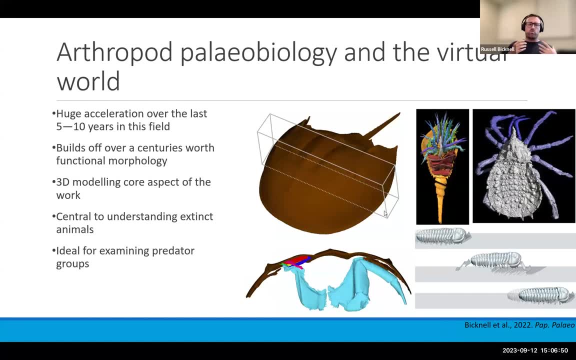 items themselves. As I mentioned before, there's a lot of really cool apex predators, especially within arthropods that arose over the Phanerozoic. When we're talking about this sort of application, we're thinking in three dimensions. 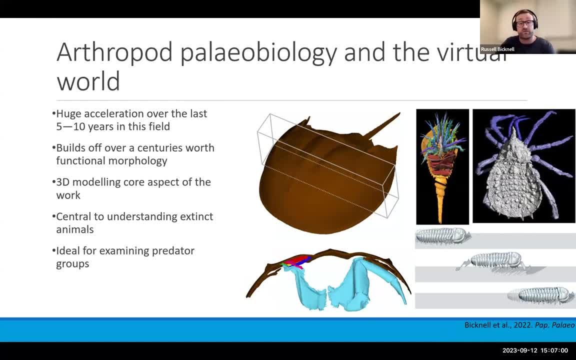 And arthropod paleobiology over the last five years, or 10 years, has seen a really amazing acceleration in terms of what we can do. So, building off over a century to two centuries' worth of functional morphological considerations, we're now able to examine our arthropods in 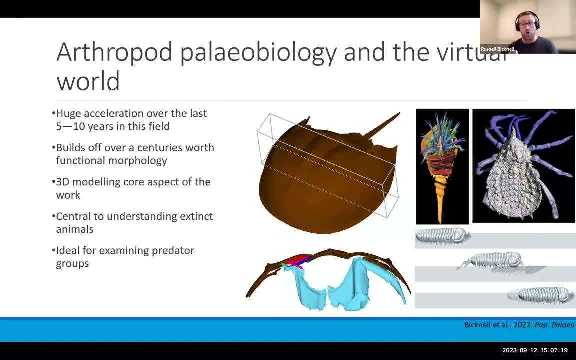 three dimensions. We're able to look at them, extract them from rock, We're able to understand how they can move, how they can function, and this framework is actually really, really ideal for understanding predator groups. So we've got this really nice shift in how we are. 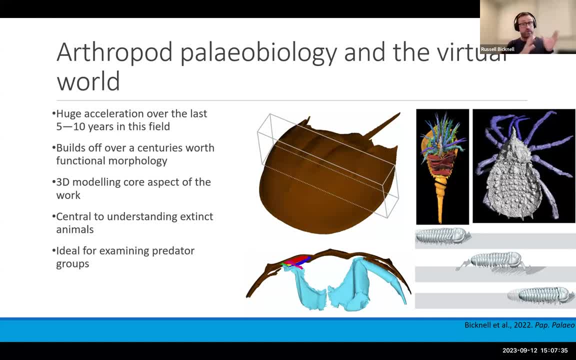 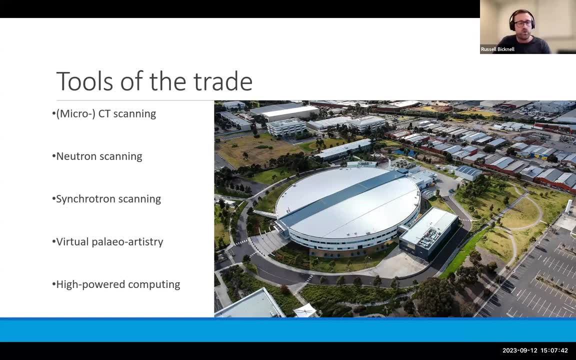 looking at predators, and this aligns with what's happening within vertebrate paleontology. So how do we do these sorts of things? Well, usually there's some kind of scanning tool that's involved. So micro or CT scanning, neutron scanning, sort of. 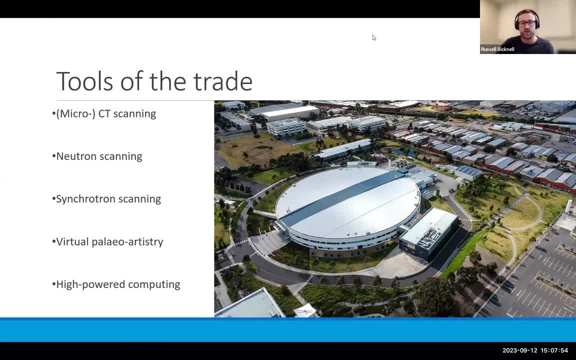 fossil and nuclear reactor or synchrotron scanning. so this is the Melbourne synchrotron. that's basically a high-powered micro-CT. we can reconstruct the animal. So if we can't scan it, if it's too pancaked or just isn't going to work, we can use paleoartistry to build the animal in. 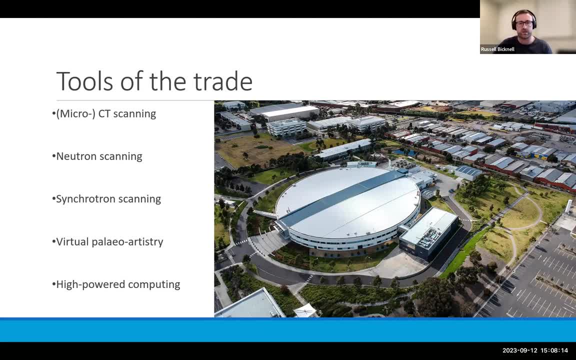 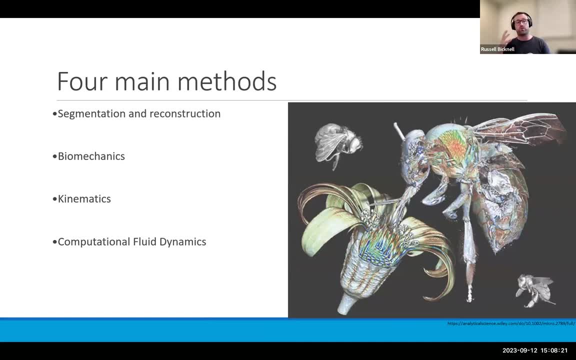 3D, And usually there's some degree of high-powered computing that goes on. So, off the back of those methods, we have four main, I suppose, approaches that I'm going to really be talking about that I've used So segmentation and reconstruction, so working. 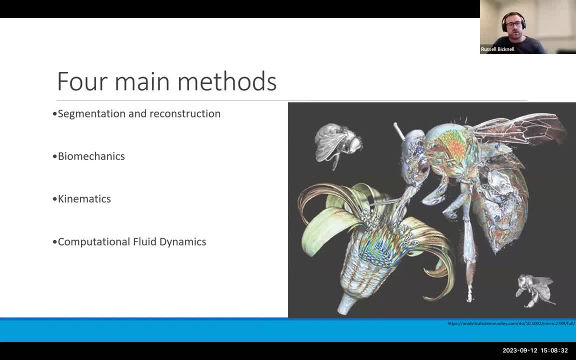 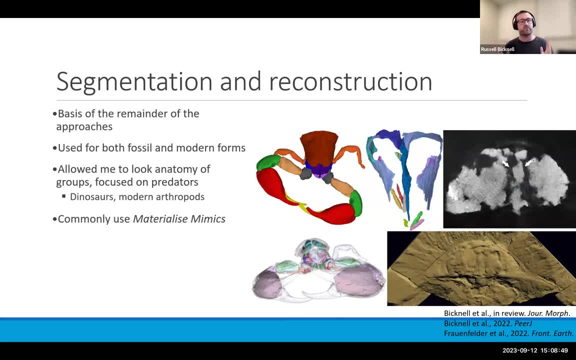 the, the bare bones, what's required to do everything else that I'm going to be talking about today, The work that I've done. I've looked at both modern and fossil forms, So this is a scorpion here and I looked at segmented scan and segmented the muscles in that scorpion. 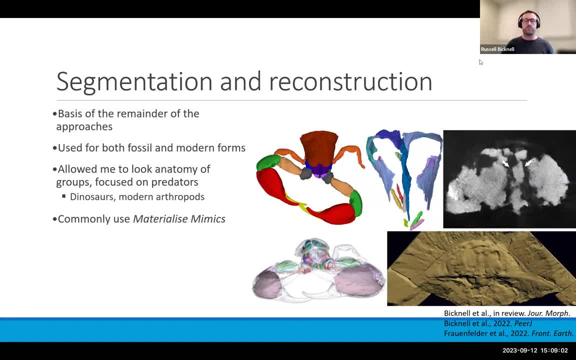 This is part of a dinosaur and this is a horseshoe crab. When we're doing, when we're scanning and reconstructing animals, we are given some really good insight into the internal structures that we're seeing that we can't often observe on the surface of the fossil, And this avoids us having 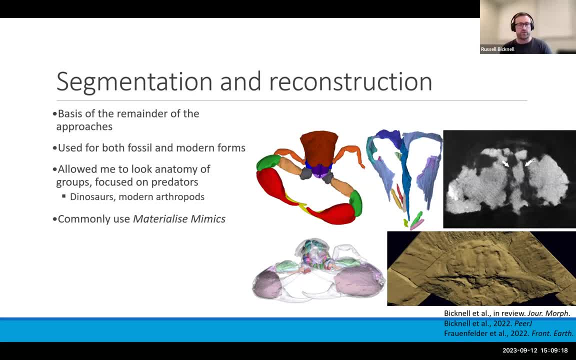 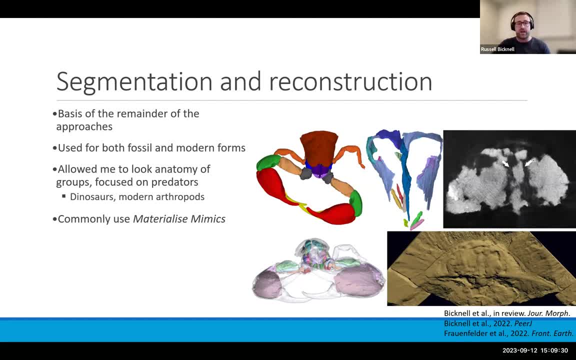 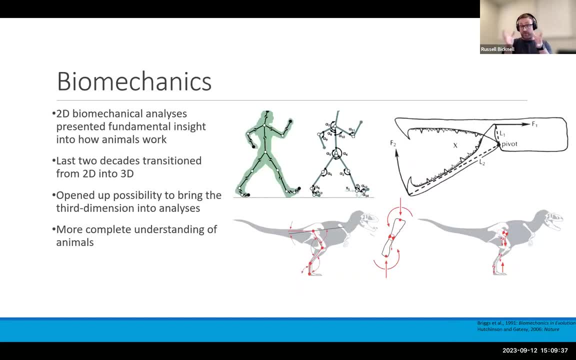 called materialized mimics, although there is an array of softwares out there that people have been using over the last 10 years. Thinking now about so with that framework there, we'll think about biomechanics. So two-dimensional biomechanics presented a really 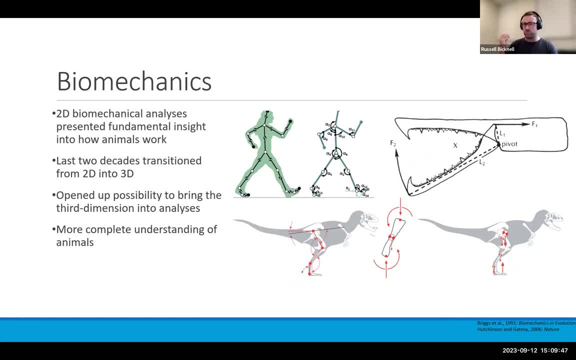 core insight into how animals function, how things move relative to other segments and how different parts of an experience force. The last two decades are a transition from two-dimensional considerations- so some examples here- to the third dimension, And so once you open up that possibility, there's a whole host of analyses and considerations that we can make. 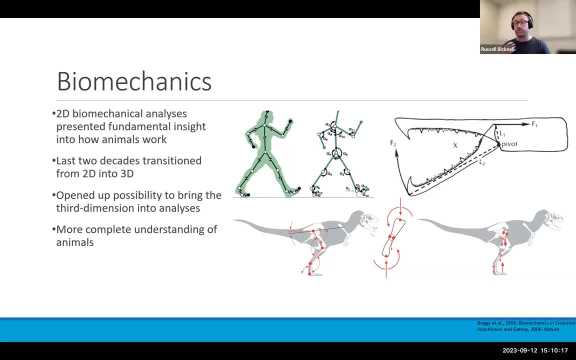 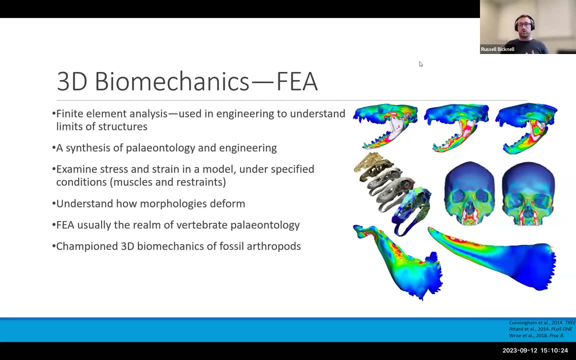 in that framework And in my view it allows for a more complete understanding of the animal in general. The tool that's most commonly used for 3D biomechanics is called finite element analysis, FEA. FEA originally was designed as an engineering tool to understand effectively the limits on a 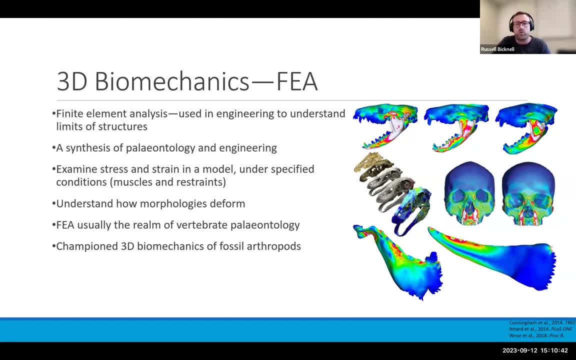 structure. So if you build a tower, where is this tower likely to collapse if it experiences an earthquake? There's been a really nice synthesis between this engineering aspect and biology and paleontology to produce three-dimensional biomechanics. This method allows us to understand where a model, a three-dimensional construction, will. 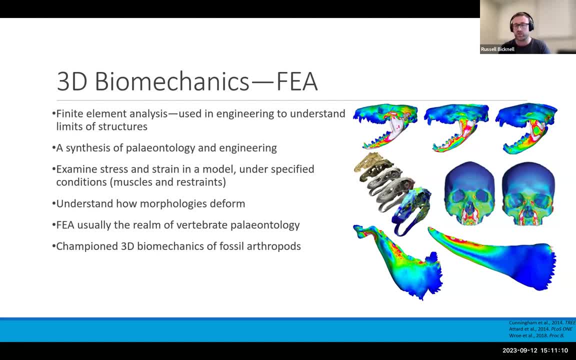 experience stress and strain under specified conditions, such as muscles and restraints. points of rotation. It allows us to understand where a model, a three-dimensional construction, will experience stress and strain under specified conditions, such as muscles and restraints. points of rotation. It allows us to understand where a model, a three-dimensional construction, will. 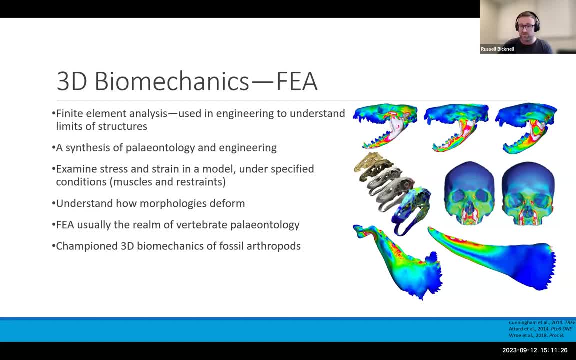 How mythologies deform. under these conditions, The majority of applications of this method have been within the realm of vertebrates. Majority of examples here are things that have endoskeletons, And so a lot of the work that I've been doing has been trying to pull our consideration of 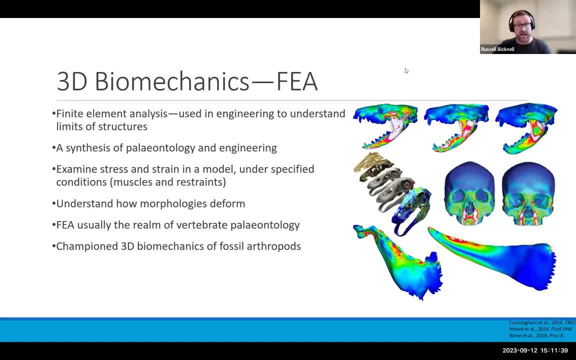 arthropods in line with where the vertebrate realm is currently at, which is really exciting. So I'm going to give a couple of examples here. I have a group of so I've got a group of protein animals and I've got a group of yeast groups that have been there for half a year that are getting 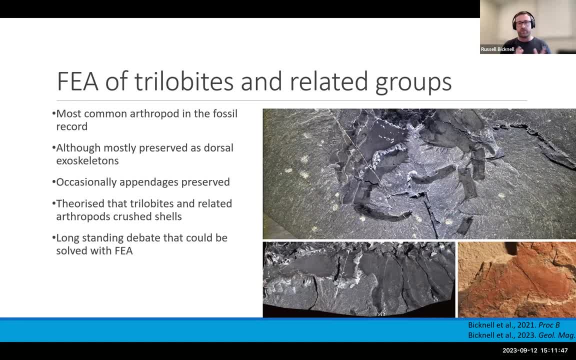 examples of work that I've done in this context. So we'll start with trilobites, because trilobites are amazing. Trilobites are related groups, things called artiopodents. Trilobites are probably the 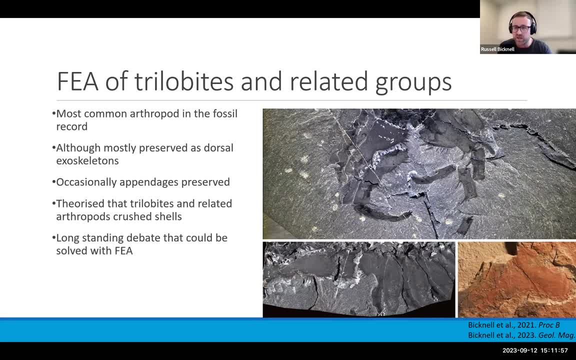 most common arthropod in the fossil record, maybe except for insects, but they're probably the most well-known And they preserve really well because their dorsal exoskeleton is made effectively of rock, which means that they are like shells. They preserve really well within the fossil record. 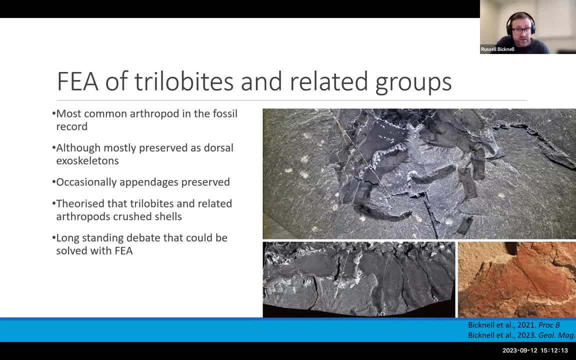 Very occasionally, though, we get the appendages preserved. So this is a couple of examples of appendages. So this is Ollanoides serratus from the aforementioned Burgess Shale. These are the leg sections there. And this is Redletcher Rex from the Emu Bay Shale. These appendages look. 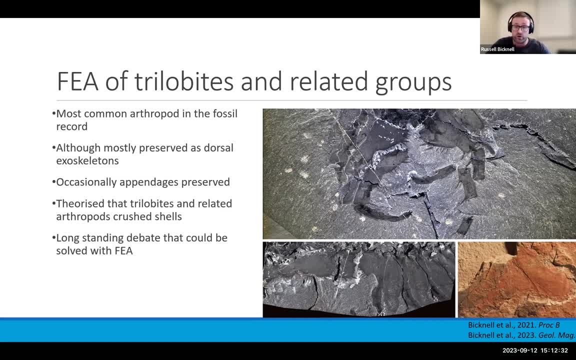 pretty similar to appendages of horseshoe crabs, And so it's been proposed that these animals were capable of crushing shells or, at the very least, eating with these sorts of structures, And so I was able to actually address this particular topic using FEA. 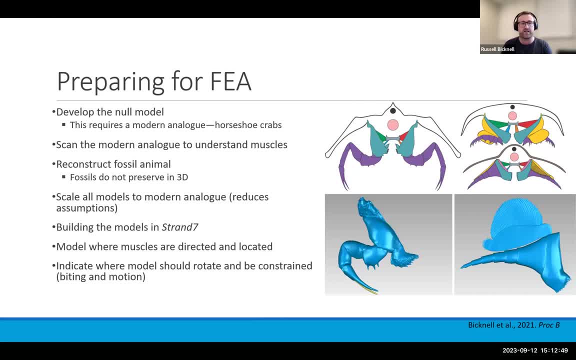 So when we are going to step into doing some kind of finite element analysis, we need to have our model, We need to have a thing we can say: well, this is a modern analog that we think our animal probably functions like, And so in this case, we chose horseshoe crabs, some lovely horseshoe crabs. 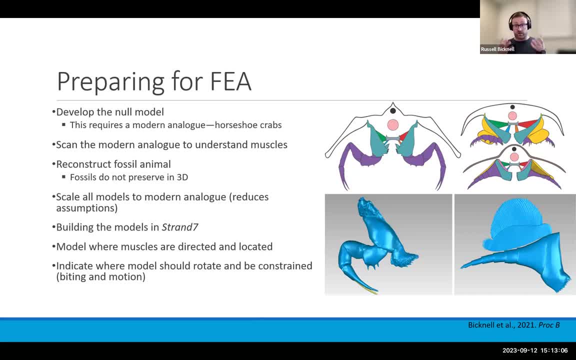 there In this case, because we actually have horseshoe crab specimens that are three-dimensional, we can put them in a micro-EC, And so what I've done there is scanned the leg, And so from there we can also determine where. 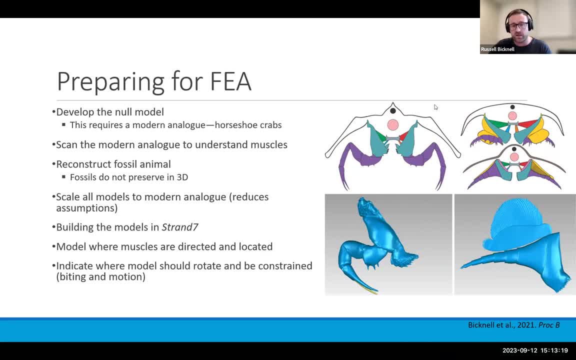 the muscles that are used in mastication are. So these little aspects here, these are our drawings of the muscles that we assume are probably going to be in our fossil animals as well. So these are one of the assumptions that we need to make. Don't make these assumptions. 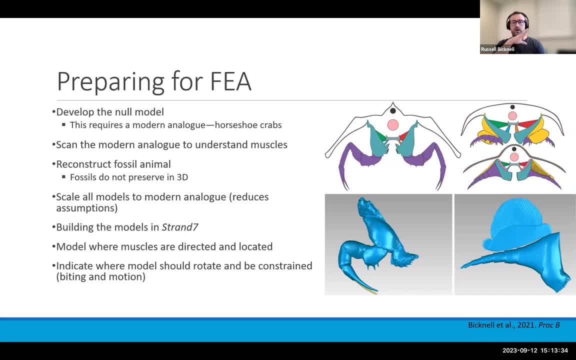 the models don't run or they don't make sense. The flip side of things, looking at the fossils, is these animals are preserved as two-dimensional impressions. They're basically pancakes And so, no matter how hard you try scanning, this is not. 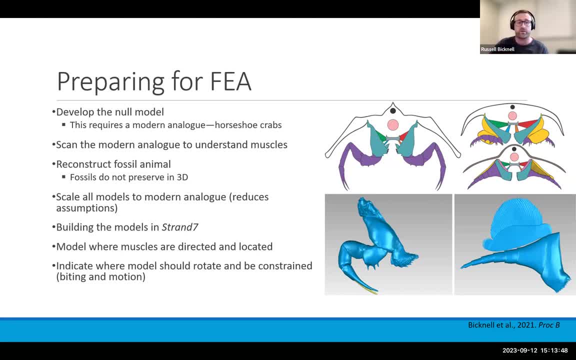 going to work particularly well, So we needed to reconstruct them in 3D. So, by looking at the fossils and comparing them in different orientations where possible, we're able to build these sorts of three-dimensional models, as you see down here, that we can then analyze. 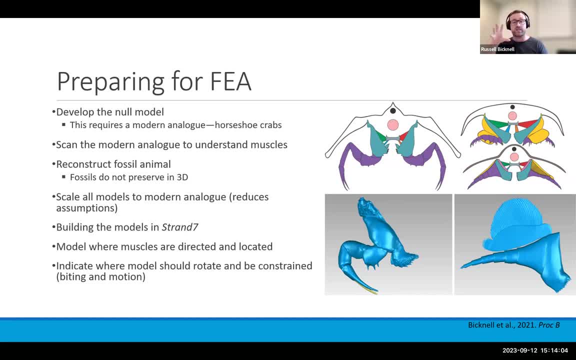 In this case, when I, before I ran, built our models, I scaled all of our reconstructions, our fossil reconstructions, to the size of 3D. In this case, when I, before I ran, built our models, I scaled all of our reconstructions, our fossil reconstructions, to the size of 3D. 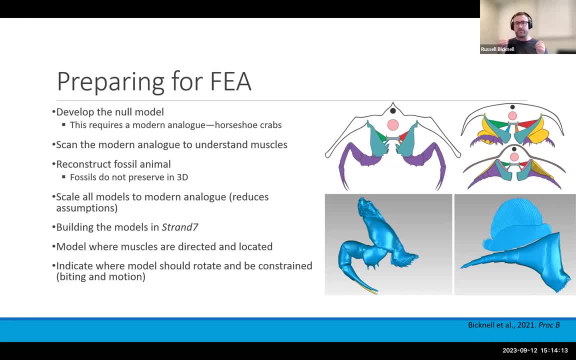 of our horseshoe crab, just because it allows us to have a more one-to-one comparison in this case, And using our horseshoe crab base model there and comparing it to our fossil things. I was able to build these models in Strand, in which case I assigned muscle orientations. 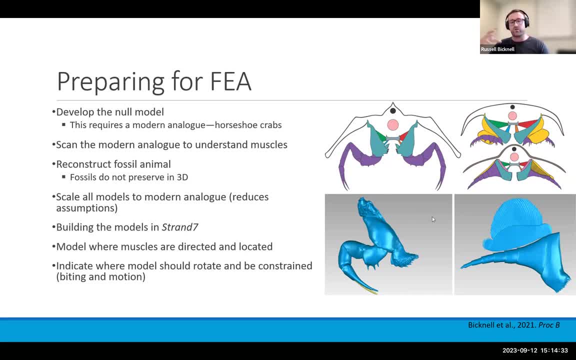 muscle sizes based on our modern horseshoe crabs, and then indicated where the models should be constrained. So in this case we know that horseshoe crabs use these little teeth here for the chewing, so we can strain those points and we know that they rotate about this point in 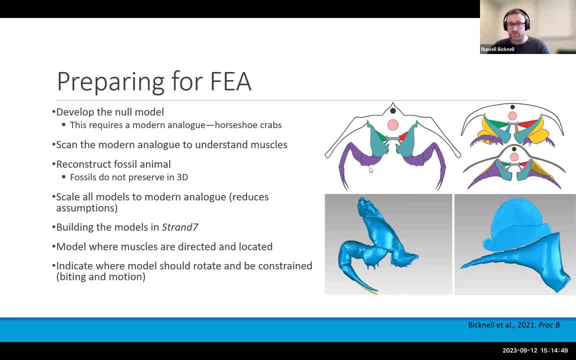 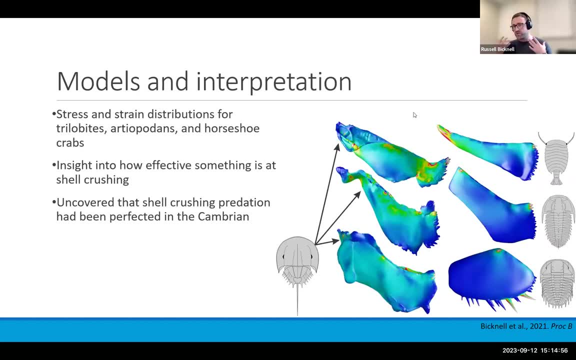 the appendage, and we effectively did the same thing for our trilobites, making the assumptions that trilobites probably function the same way that horseshoe crabs do. What does this all do? Well, it produces a really nice array of pretty, pretty colors. It allows us to see where the 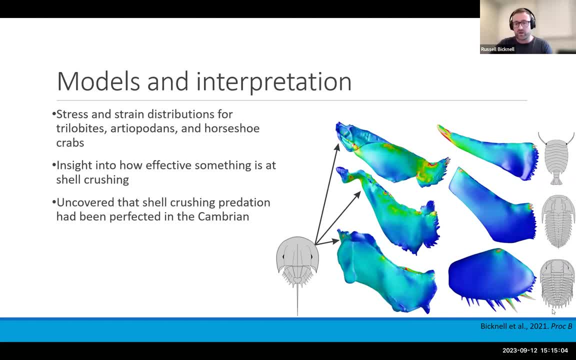 stress and strain distributions of trilobites, these two here, artiopods- this is Sydney- and Expectans I mentioned beforehand, and horseshoe crabs in the models And we can see that our horseshoe crabs and Sydney have a very similar color distribution. stress-strain distribution. 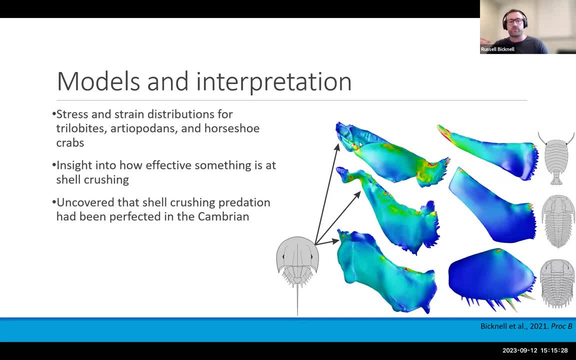 which tells us that Sydney is probably similar to horseshoe crabs in terms of how it can crush shell, which makes sense because we've seen examples of Sydney with shells in the gut content. Looking at our red-lithered rex here and all of the serratus. 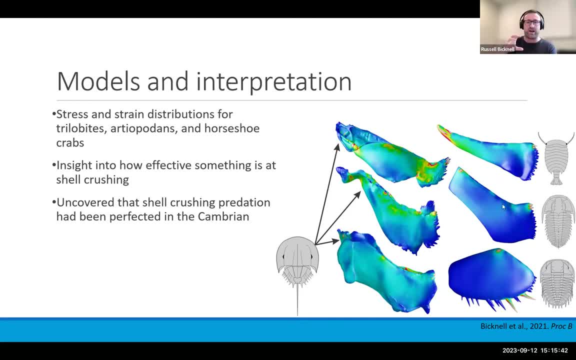 there's a lot of blue. this tells us that there's limited stress strain experience through the model and we think that for red literature this indicates a more effective construction for shell crushing, because it's got little stout spines there and it really does look like a. 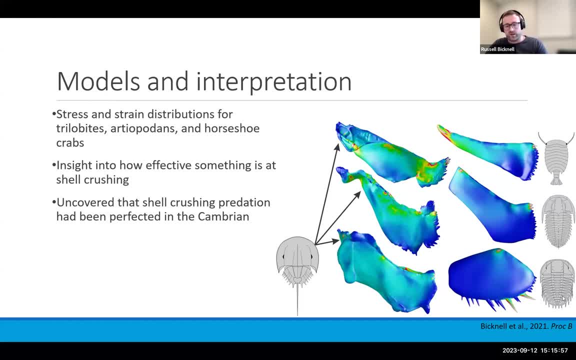 nutcracker of an appendage, uh, olinoides, on the other hand, has these really long spines as they elongate structures there, and we think that the majority of the stress is actually taken up in those spines. and so if this animal were to try and tackle, say, some kind of shelly organism, 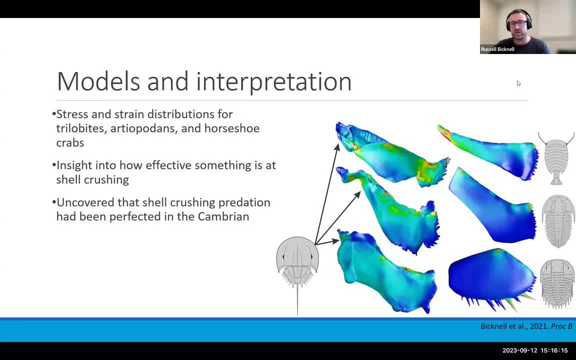 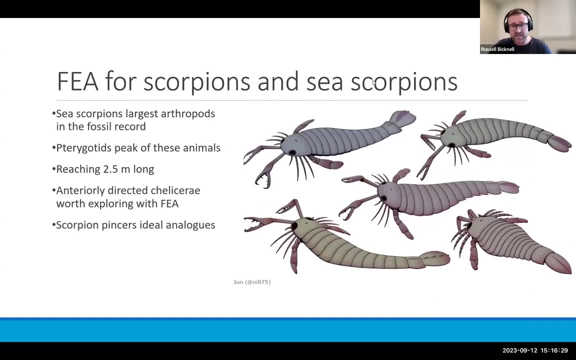 like another trilobite, it probably would have experienced failure along those spines. so this gives us some really good insight into what was doing predation at the cambrian, a really important period of time in which life was really taking off. my second example today is sea scorpions. i. 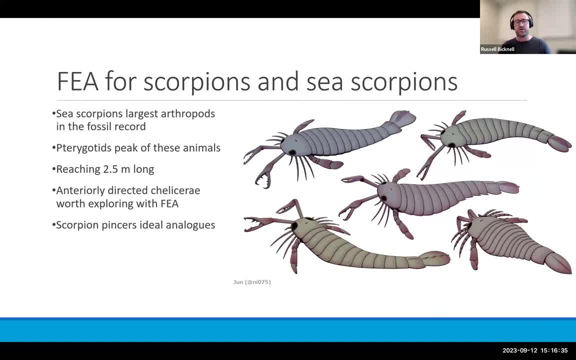 love sea scorpions because they are amazing, they're really large arthropods. they're really what happens when you just you, you take, you take an arthropod and you just push it to its logical extreme and you get two and a half meter long. 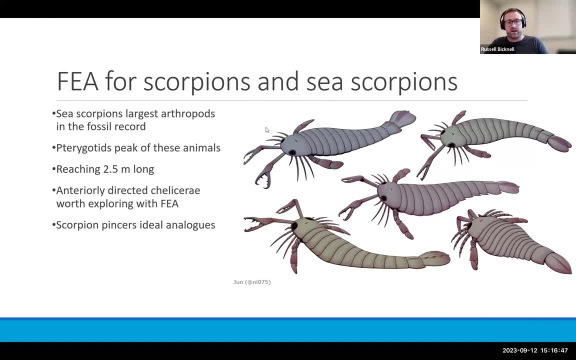 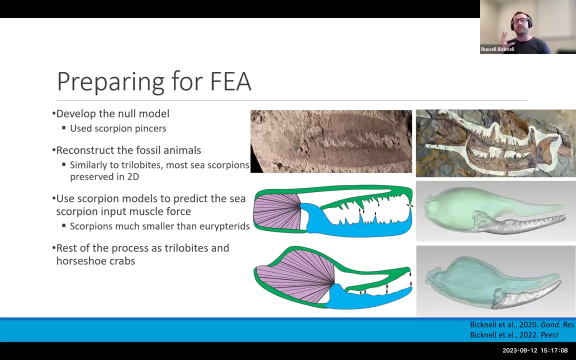 beasts and they have these really, really amazing, uh, modified chelous racer, anteriorly directed grabbing structures. these look very similar to scorpion pincers and so means that we had a really ideal comparison to understand scorpions versus our sea scorpions. the construction for this approach was slightly modified from what i did with our trilobites and our horseshoe crabs. once again, we start with our normal and our model is that sea scorpions probably function like scorpions and from there we scan- i said scanned- a bunch of scorpion pincers and had worked with colleagues across the world who'd previously done similar work- our sea scorpions. 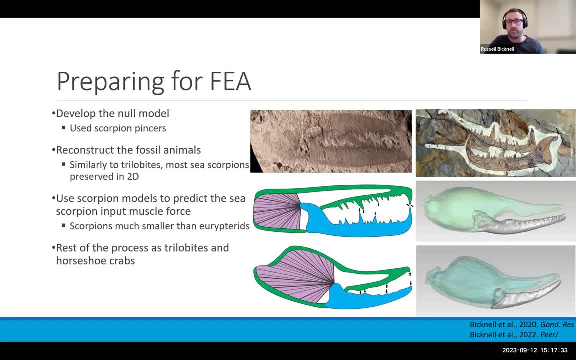 on the other hand, we needed to reconstruct again because, similarly, trilobite appendages- sea scorpion, chelous right- are for the most part preserved as two-dimensional impressions, so scanning it's not really going to work so well now, as opposed to scaling, uh, the trilobite models to the size of the horseshoe crab, which is what i did previously. in this case, we actually used our scorpion muscle, scorpion models and muscle sizes to predict how forceful our sea scorpion pincing force would have been and the reason we did that. 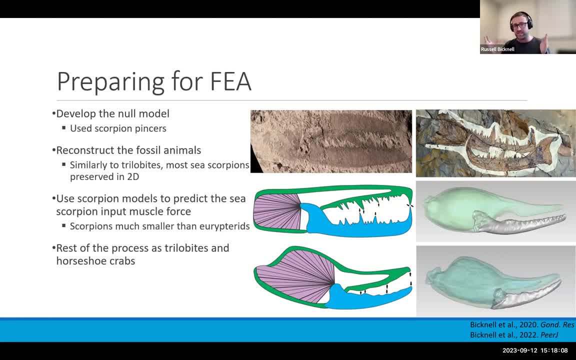 is because we don't want to scale our two and a half meter long beast down to the size of a scorpion. um, there are complications that arise from that, and ultimately it's not a very realistic representation of these sorts of animals. uh, other than that, though, the 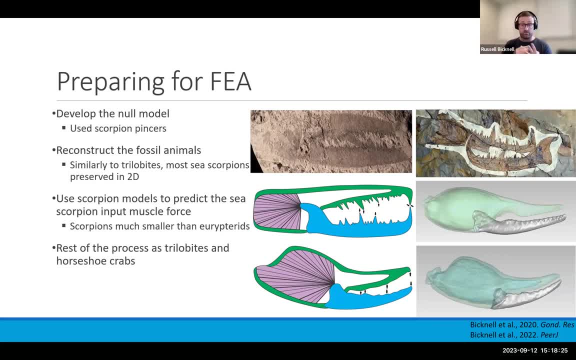 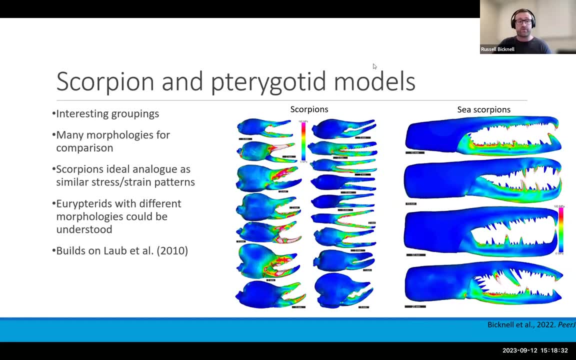 rest of the process was the same: um, scan, reconstruct, work in mimics- uh sorry, uh- work in strand and then resulting models. so we have our scorpions and our sea scorpion models here. so what's really funky with this is we were able to look at scorpion groups as well as our. 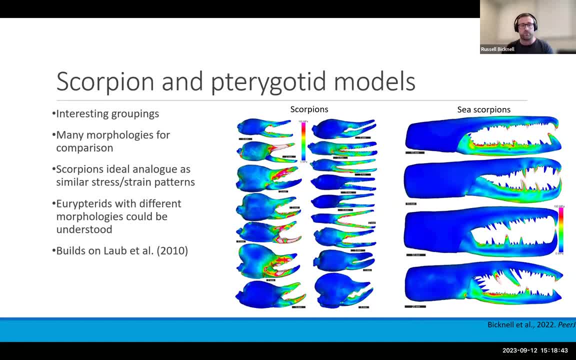 sea scorpion groups and compare and contrast between the two, the fossil and the modern. and so because we had so many different morphologies and scorpions, we had an ideal range that we could compare to, and we see that in generally speaking, that the stress strain distributions in our 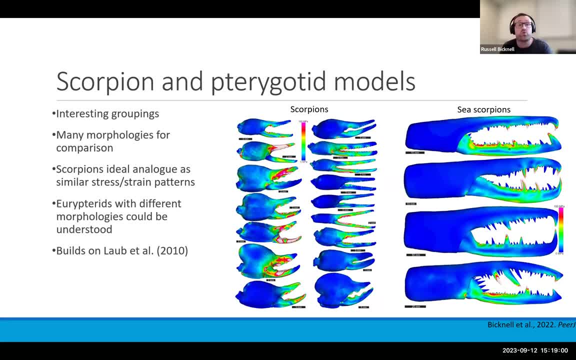 scorpions is similar to rc scorpions. this probably was a pretty good choice of a comparative model there, which is ideal. we were also able to then focus in on our c scorpions to understand what those different morphologies actually represent and what they mean in the context of stress and strain. so we 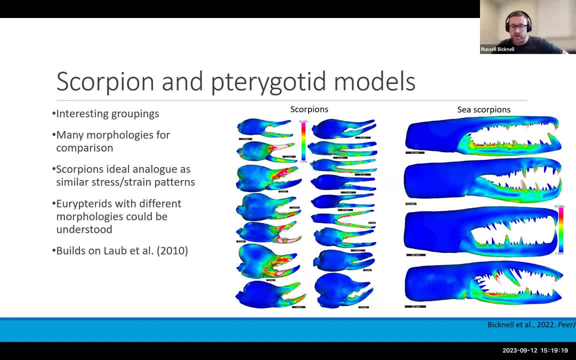 can see here we've got uh forms with more elongate spines here that probably were less effective at really dealing with reinforced prey, especially um acute ramus over here, which has really inclined serrated morphology that we can see the areas of high stress there would have really experienced. 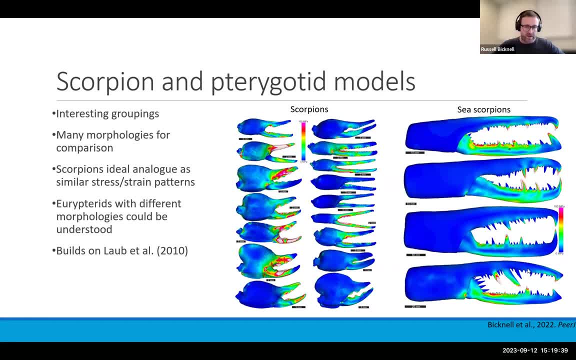 some, some pain if it were to try and grab down on something a little more reinforced. uh. by comparison, a jacaloptera csa, that is, the two and a half meter long uh animal, has generally lower stress, a lot more blue, along the model, telling us that this animal was a lot more. 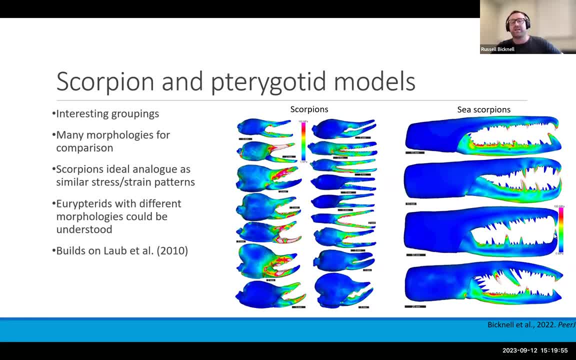 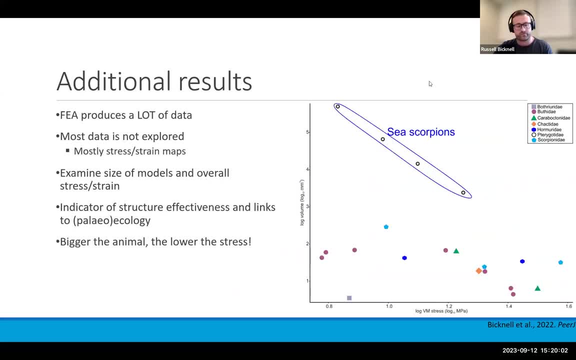 reinforced with those lovely stout spines, meaning it was probably more effective at targeting prey items that were more reinforced. now the finite element model is a very good sample of those different morphologies in our model. so I might take a look at that in a moment and I guess i'll kind of comment a little bit about the different morphologies of the different morphologies in our model. 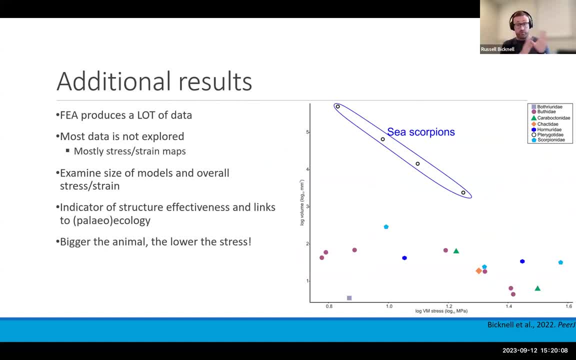 models produce a ton of data, Like they really do make a lot of data. I'm showing you figures, but that's based on a lot of information, And so we can actually pull this data out and more further contextualize our models and our animals. So this is what I've done here. I've looked at 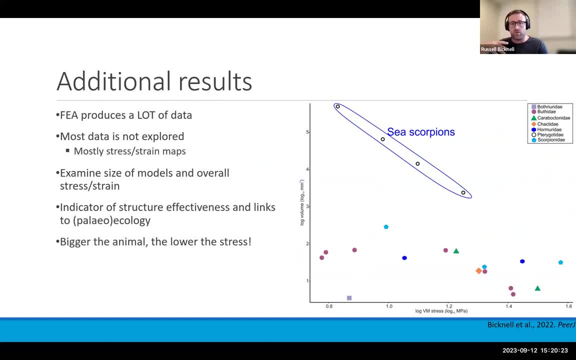 the vomitus stress. That's effectively an overall measure of how much, how blue or how red our model is, And I've looked at the volume of our models, So how much space our models actually show, And what we can see is that as your animals increase in size, so as you get to that, two and 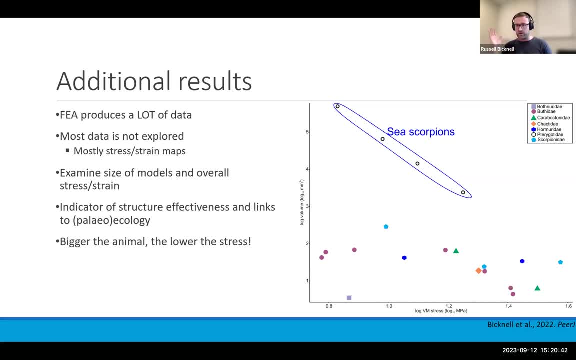 a half meter long interval, you generally experience lower stress and therefore you're more effective at using these structures, at grabbing and dealing with prey, which is really quite cool. And finally, we can think about these animals in the context of phylogeny, And so we can. 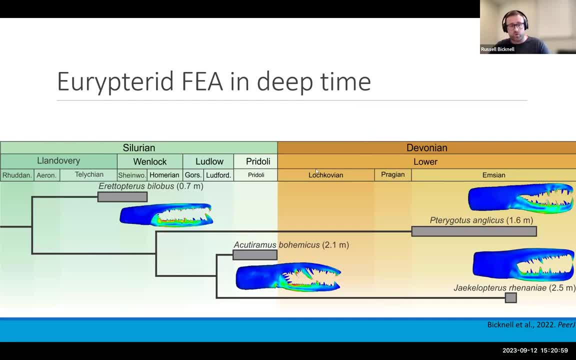 see that phylogeny in time, And so we can see that as we move towards Silurian and Thetavonian, we're moving towards It's modern day. There's a transition away from these sorts of, I suppose, more inclined morphologies. 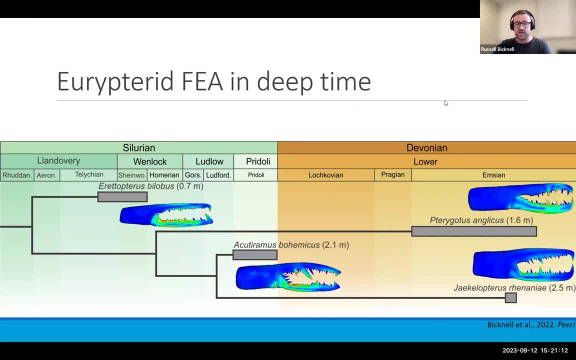 into a more stout-like structure that we see in Pterygodus and Yagalopterus. This could be associated with the rise of armored fish and then a transition for sea scorpions sort of to be more effective predators dealing with those sorts of prey. All right, So let's put biomechanics aside. 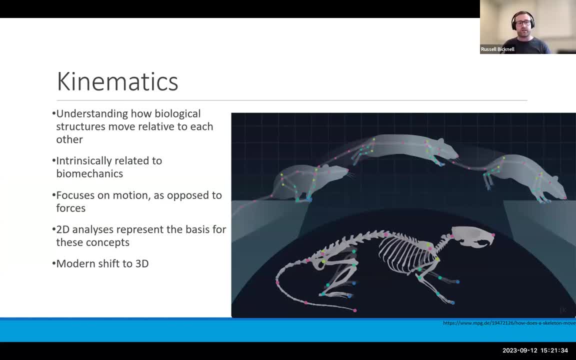 for a second. Think about Kinematics. Kinematics is effectively a method that allows us to understand how structures move relative to each other. Intrinsically, it's therefore related to biomechanics, but it focuses more on motion, how things move, as opposed to the forces things can experience. The majority. 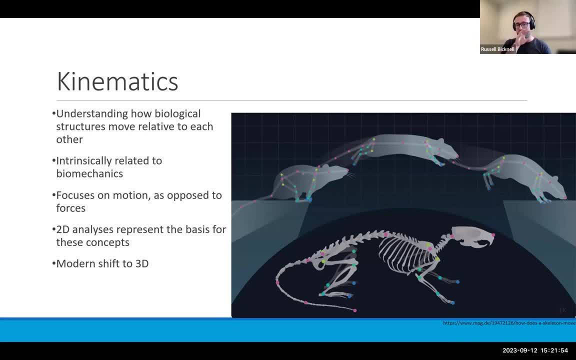 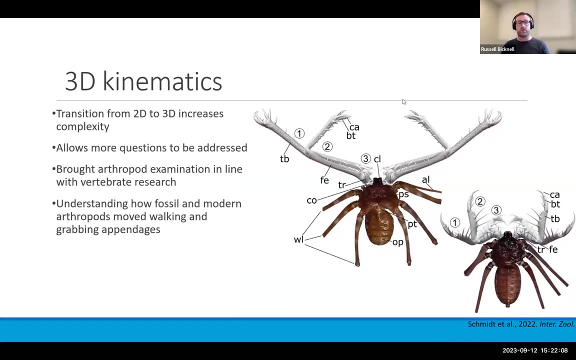 of work that's been done with kinematics has once again been in the two-dimensional, but a modern shift to 3D, also within the vertebrate realm, has allowed us to start thinking about these animals, animals in general, in that bigger context, which is really exciting. So work that. 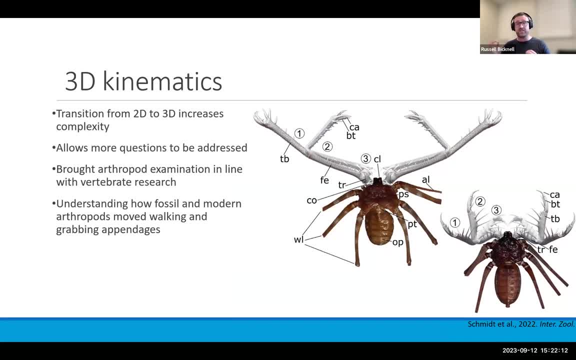 I've been doing with colleagues across the globe has started to look at 3D kinematics of arthropods And in particular we're looking at things like chelicerae, things with large raptorial, anteriorly directed grabbing appendages. We've got sea spar, excuse me, We've got. 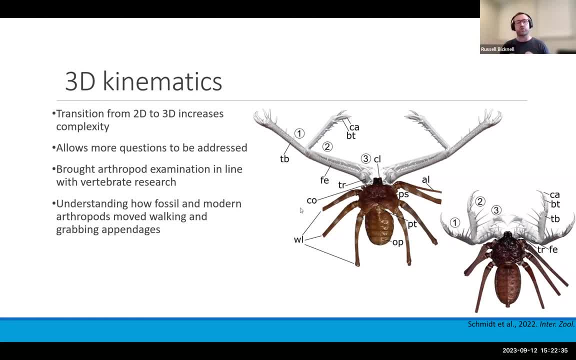 a couple of chelicerae here with those large grabbing appendages And we can also look at. so we can look at how they move and we can also look at the walking legs of these animals. We can look at how these animals are able to walk and compare them to both other modern forms and also 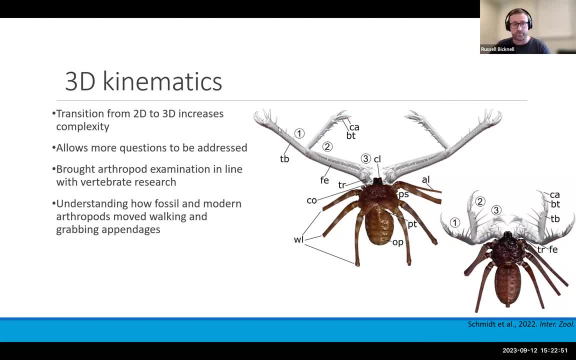 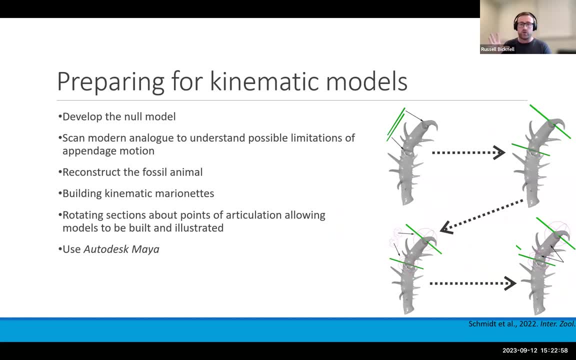 specimens, species in the fossil record, where possible. So how do you build a kinematic model? Well, once again, you start with your null model consideration. So if we want to look at something that has a large grabbing appendage in the fossil record, we want to look at something. 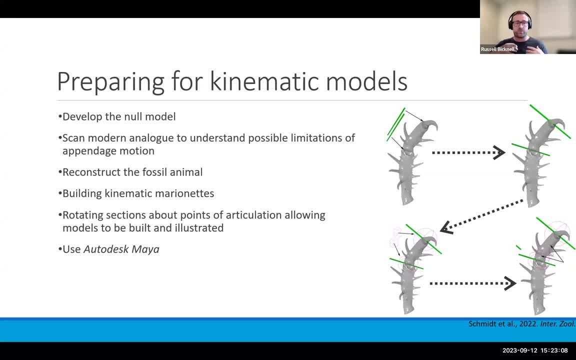 in the modern day that does have that, And so examples that I showed you there are of some arachnids that have those large anteriorly directed grabbing appendages. We scan usually our model because allowing that allows us to then segment out those main. 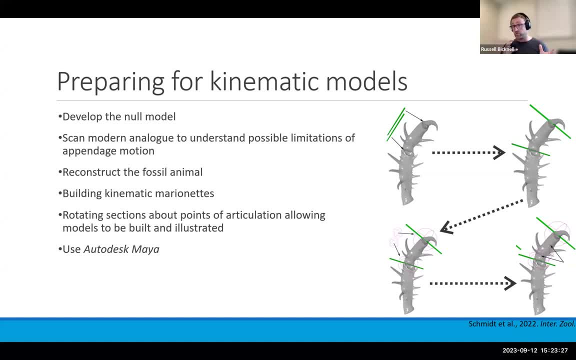 different exoskeletal segments and then to understand the possible range of motion that this structure, this animal, could actually experience. Generally speaking, we'll have to reconstruct our fossil model. similar problems as before with our biomechanics. These animals are often preserved as two-dimensional impressions. 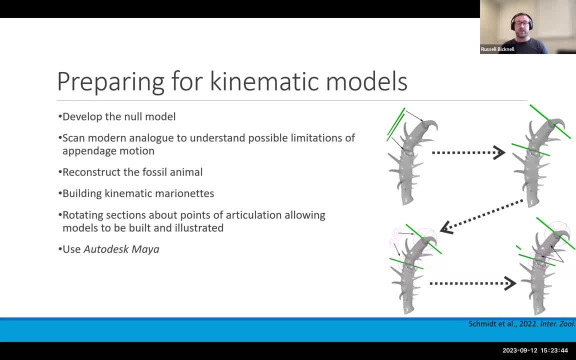 which limits how much we can scan, And then we'll build our kinematic marionettes. So what that means is basically this is what this pathway is showing you here. We'll build that step by step. This is what will move relative to the next subsequent part of the exoskeleton, And by rotating these differences. we can then build our kinematic marionettes, So we can build our kinematic marionettes. So we can build our kinematic marionettes, So we can build our kinematic marionettes. And then we can then build our kinematic marionettes, So we can build our kinematic marionettes. 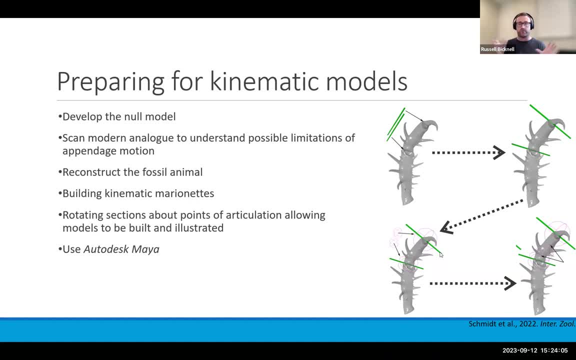 segments, as we're doing here, we'll be able to figure out the full range of motion for the entire appendage. In this case, the software that was used was Autodesk Maya, although I think you can now do it in Blender as well, which is really cool and also Open Access and free. So let's 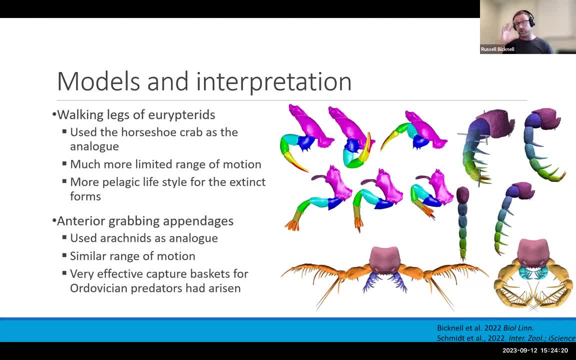 think about a couple of examples here. We're going to first look at walking legs, then we're going to look at those grabbing appendages, sort of thinking about those large arthropods, once again the fossil record, So sea scorpions, eurypterids, some of them have a lot of 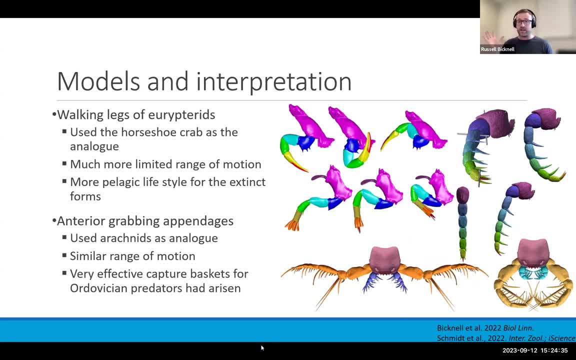 these large anteriorly directed grabbing appendages. some of those have those large chelicerae that we saw before And they also have walking legs. So this is a reconstruction of the walking legs of eurypterids, probably the most iconic sea scorpion, And we compared this to 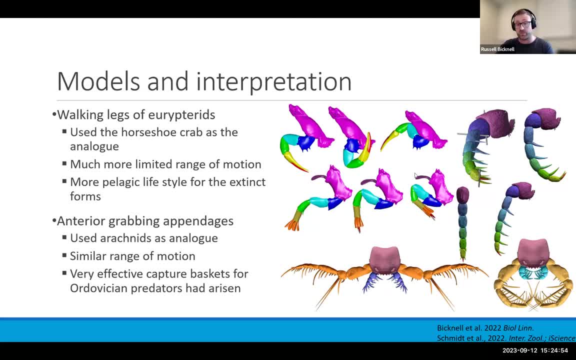 the walking legs of horseshoe crabs and it's also pushing legs of horseshoe crabs as well, Because we kind of figured that at least horseshoe crabs and sea scorpions are related to each other And it's been proposed that these animals probably did walk, functionally similar to. 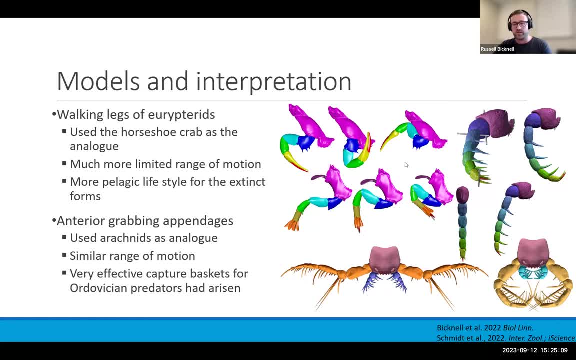 horseshoe crabs, And what these models show you is that our horseshoe crabs have a lot more range of motion. They can do a lot more with their walking legs and their pushing legs than sea scorpions, our eurypterids, can, And so this really aligns with the more pelagic life mode that we. 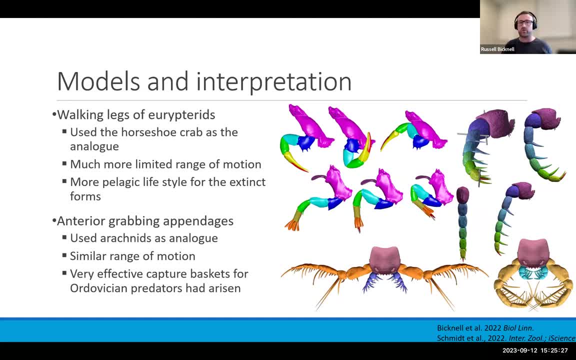 think our eurypterids had So swimming around as opposed to scuttling on the sea floor. Then thinking about our large, anteriorly directed grabbing appendages, using those arachnids as the modern analog, once again, we can see that there's a similar range of motion, from fully outstretched to effectively. 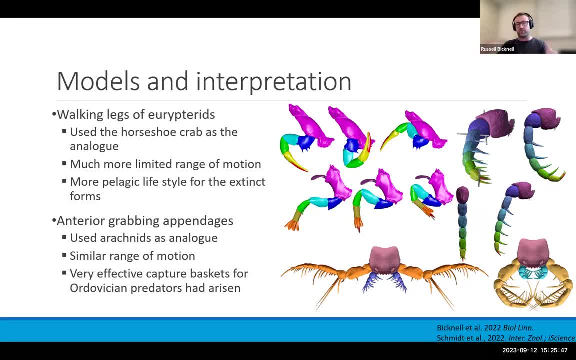 fully enclosed, developing what's called a capture basket. And so we've got these, these autovision animals, really when sea scorpions were just starting to really take off, having very effective means of capturing and then processing prey that is. 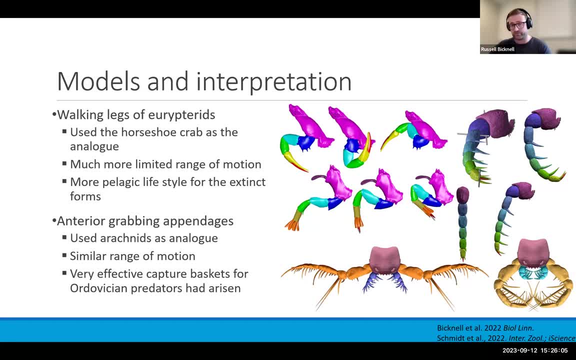 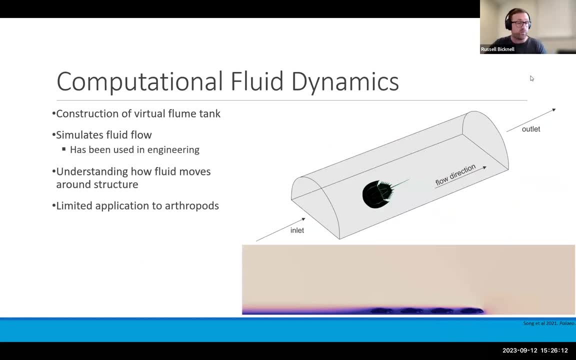 effectively being replicated in modern arachnids. Okay, so the last method that I'm going to talk to you about today is computational fluid dynamics. This is sort of the frontier of my work. CFD allows you to build a virtual flume tank. 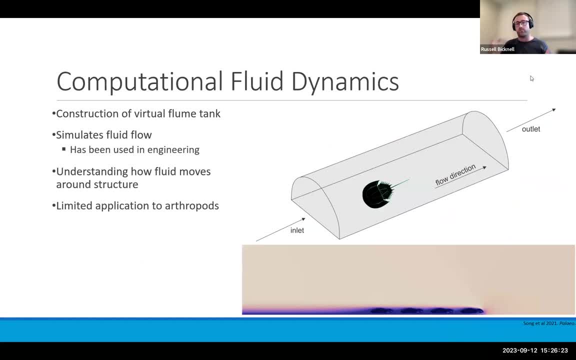 so effectively. you can look at how fluid will deform around a structure that you plonk in this flume tank. And, once again, it's been primarily used within engineering. it's been recently. it's been primarily used within engineering. it's been recently. it's been recently, it's been. 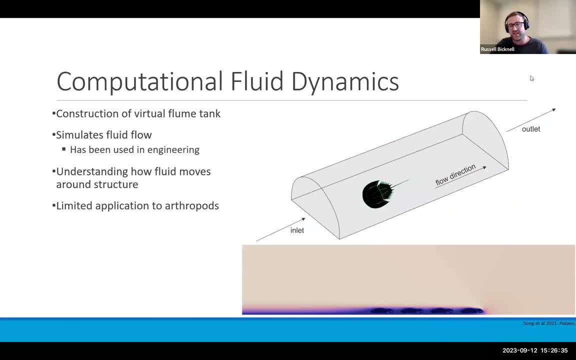 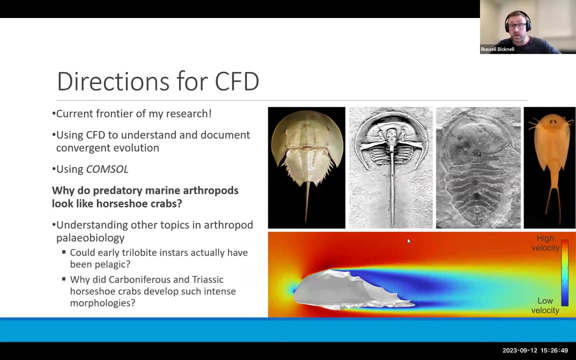 synthesized with paleobiology to more completely understand animals. So people have used it to look at arthropods, and so these are some trilobites down here, but really the application within arthropods has been quite limited. So what am I trying to do? Well, I'm trying to look at CFD to 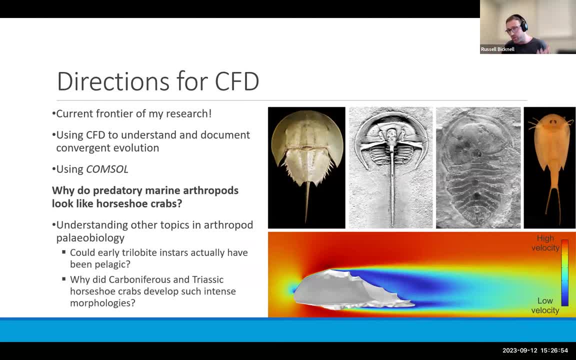 understand how and why so many arthropods end up looking like horseshoe crabs, my favorite group of animals of all time. So we've got an array of examples here. so that's a horseshoe crab, that's a trilobite, that's an arthropod that was around about the same time as during the Cambrian, and 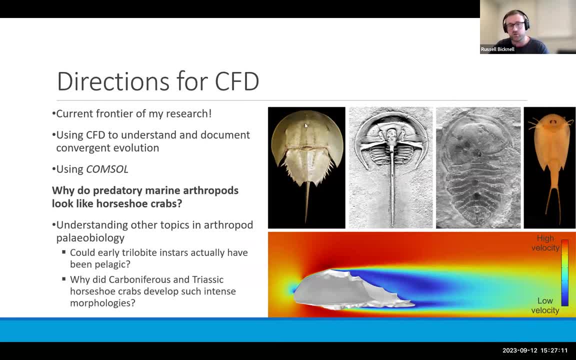 this is Triopsis, one of the modern day crustaceans that kind of looks like a horseshoe crab, And so some of the questions I'm looking to address with this basically understand, like: why do arthropods converge that live in marine environments converge on a horseshoe crab-like? 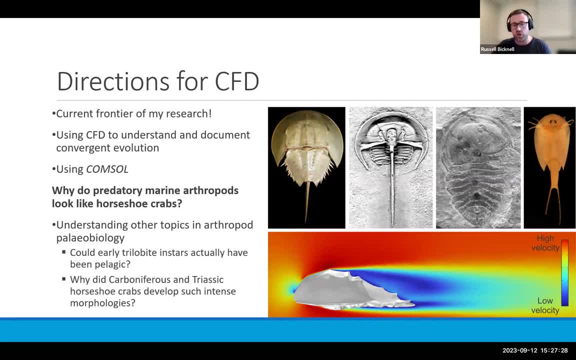 shape. Is it something to do? is this an ideal orientation shape for living in the water, or is this something else? So it's a question of why do arthropods converge that live in marine environments? I'm also planning on using these sorts of questions to address topics around. 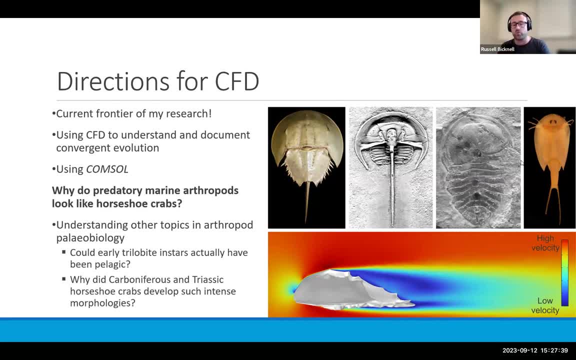 whether or not really really baby trilobites were pelagic, so could they have floated around the ocean more effectively, as has been proposed? And why do we see an array of really complex, crazy morphologies in the horseshoe crabs during the Carboniferous and Triassic? 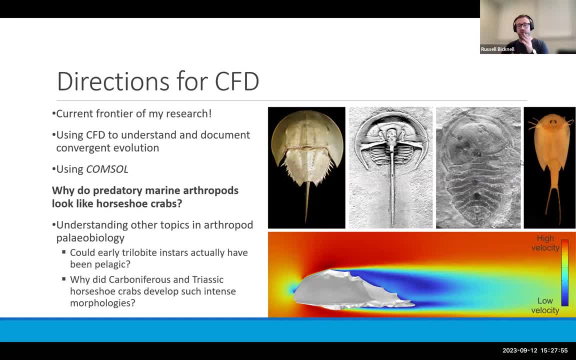 when horseshoe crabs weren't really living in the ocean, they were probably living in more sort of brackish estuarine conditions, Which means that really this model, this modeling approach, is going to allow us to tackle and more thoroughly understand arthropods in that marine context. 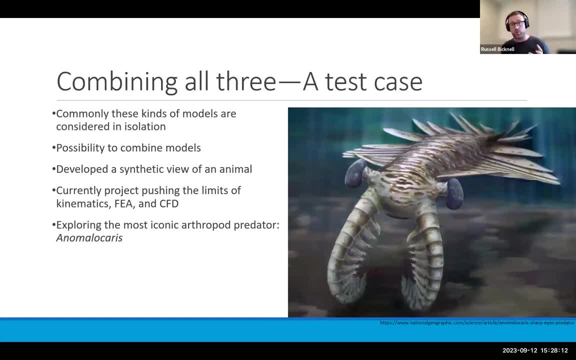 All right. finally, what if we put this all together? Okay, what if we go? okay, we've got these three different approaches plus reconstructing. What if we build something to fully understand an animal by synthesizing this together? and I decided to do this because usually 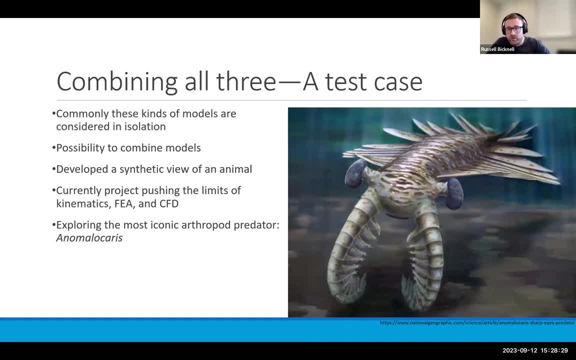 these sorts of models are considered effectively in isolation, but if we put them together, we can more thoroughly document them, document an extinct organism, And so I've done this. I focused on probably the most iconic Cambrian animal, Anomalocaris canadensis, which is thought to have been a true apex predator. 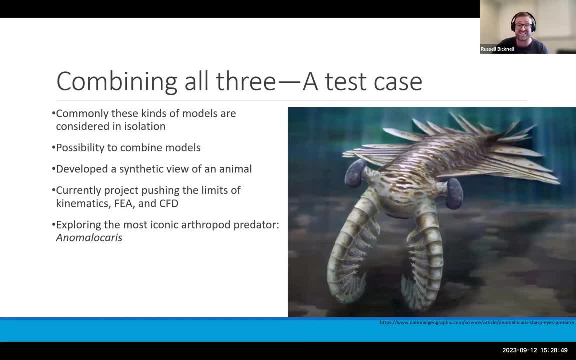 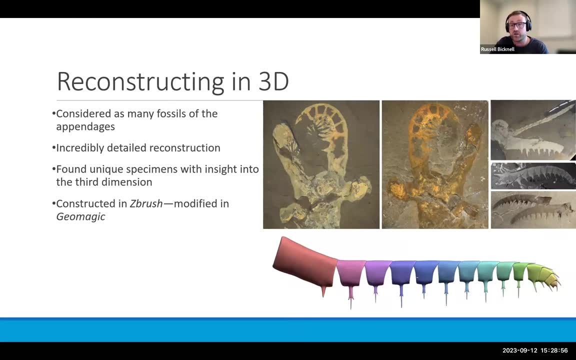 And so, by using kinematics, FEA and CFD, we were able to test this idea. So, first off, we start by reconstructing an animal. Now. Anomalocaris is so well documented in the Burgess Shale that we had 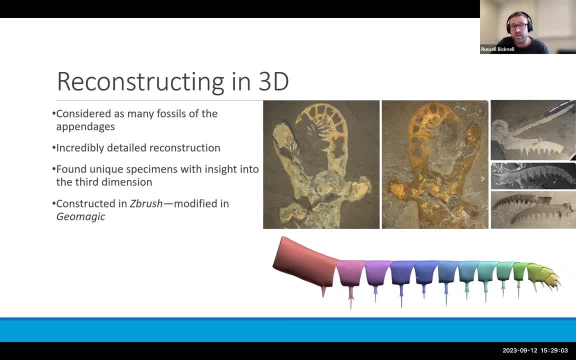 an array of orientations for the fossils that we could use to build our three-dimensional model, which is what this is In fact. this is, I think, the most accurate 3D reconstruction of this animal, And this level of accuracy allows us to really pinpoint really minute changes in the range of. 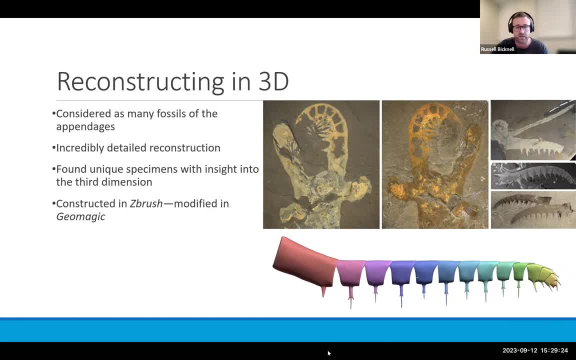 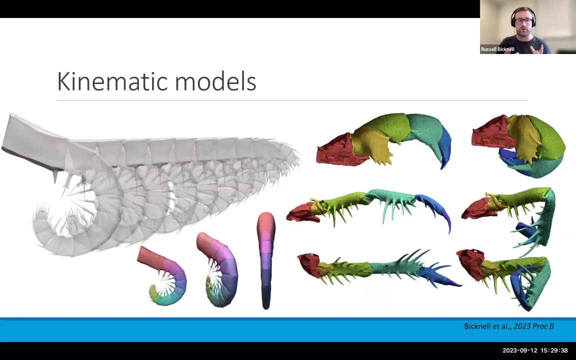 motion and then subsequently biomechanics of these sorts of structures. This particular was constructed within ZBrush and then I modified it within a program, Which are really really good if you're trying to build three-dimensional models. Then we took our kinematic approach: We've got our reconstructed animal and we wanted to rotate it. 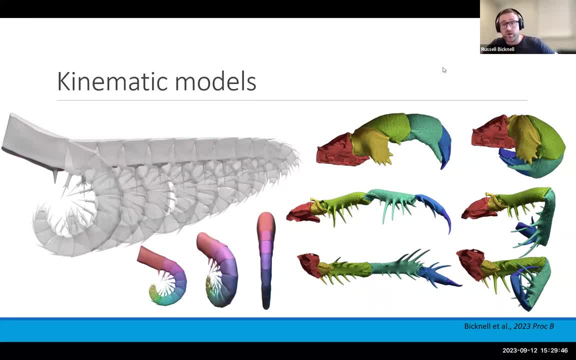 But of course we need our null models. So, once again, talking about those arachnids, with those really large anteriorly directed grabbing appendages, here's a couple of examples here. So we were looking to see, did our Anomalocaris appendage? 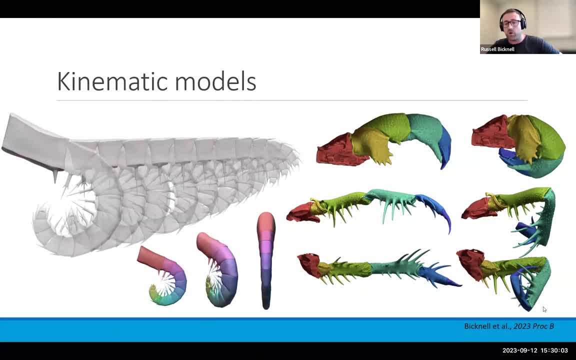 really rotate in a similar way to the way that we know that our whip spiders and our whip scorpions can do, And realistically, we did show that. So this degree of closure that we see, or openness and closure, is replicated in our Anomalocaris model, telling us that, yes, this animal did use its appendages. 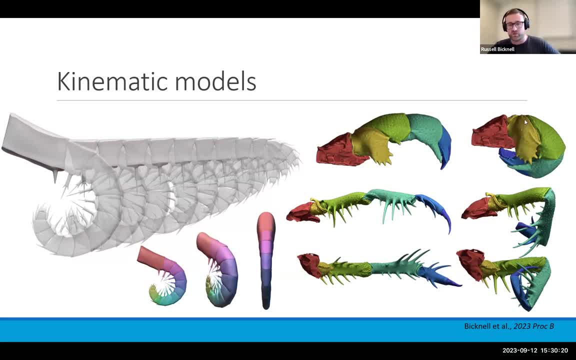 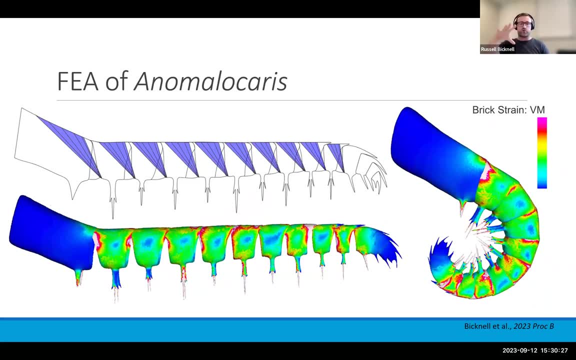 to grab, in a similar way to modern whip scorpions and whip spiders. The next step was to look at these two extreme ends of our model, so the outstretched and the enrolled condition, And then build that biomechanical model. In this case, what I had done is I had built an array of 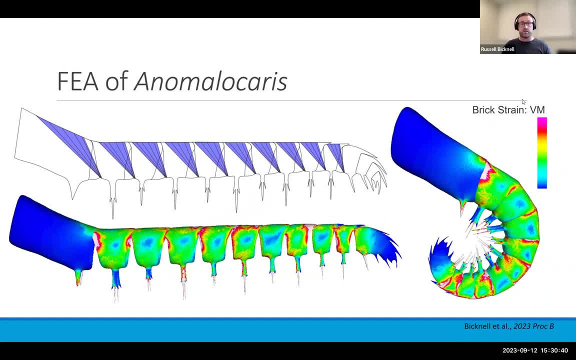 different muscles here, based on sea spiders, So we don't know what Anomalocaris muscles look like. It's one of the main limitations when we're trying to apply these sorts of methods to anything in the fossil record. But we can look at modern animals and say: how do you use your appendages? 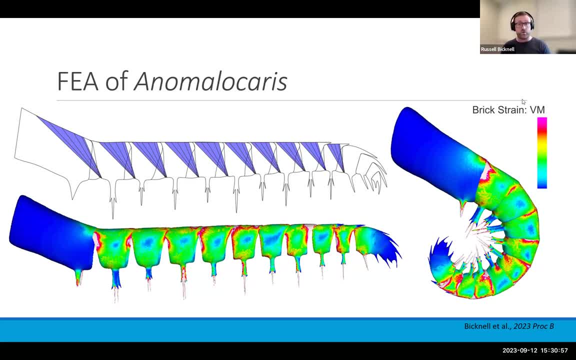 And sea spiders have this really funky adaptation where some of their appendages are used to affect their body. So we can look at modern animals and say: how do you use your appendages? And so we kind of figured that, given that the appendages are structurally very similar and the 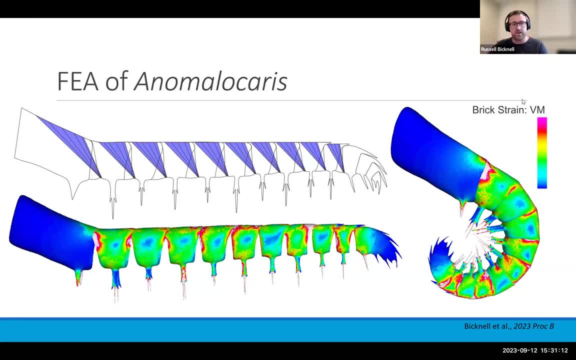 potomias. the different sections are kind of built the same, that the array of muscles we proposed here probably actually made sense, And this allowed us to see that there are a lot of areas of high strain, especially at these points at the spikes. That tells us that, well, when this animal 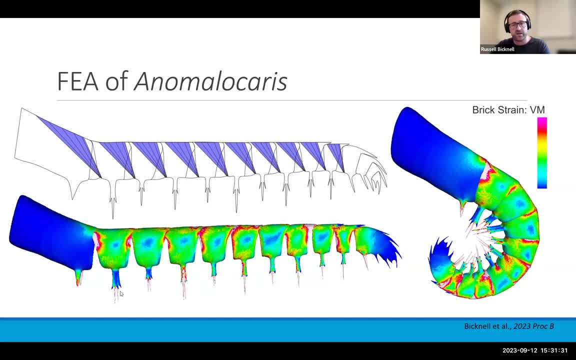 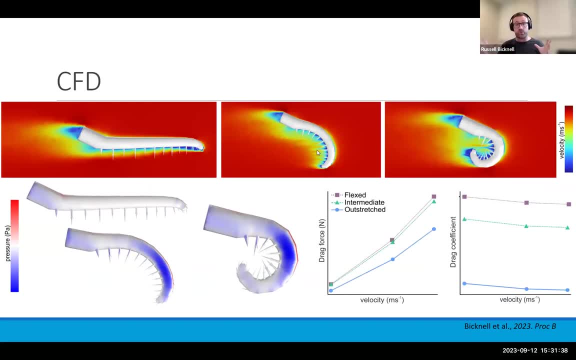 was grabbing something, it probably would have experienced a lot of strain, So we can look at some pretty high stress and strain at the tips of these spines. Then we took three different conditions- so fully outstretched, partly enrolled and completely enrolled- and placed this animal in. 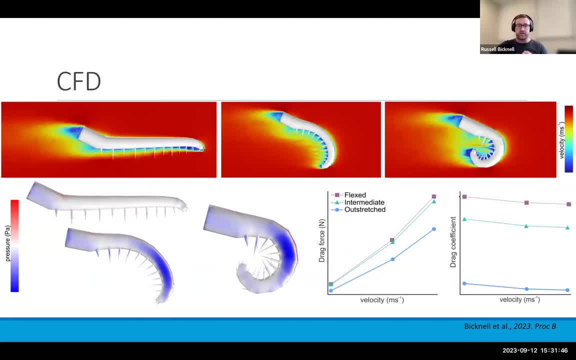 that virtual flume tank that I mentioned before, And this allowed us to understand that the most fluid dynamic orientation for the appendages was completely outstretched. So this animal probably would have been outstretching its appendages to attack and rolling the appendage. 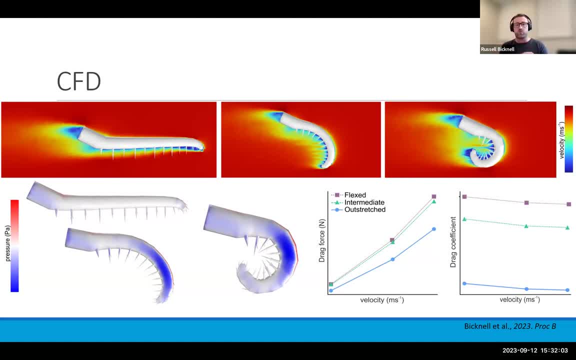 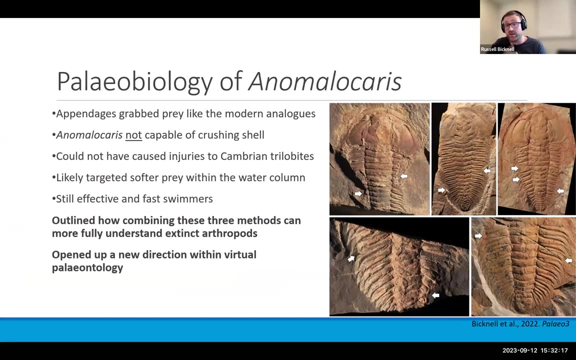 around a prey and then decelerating after that. And so with this combination of aspects, we can really fully understand how Anomalocaris was functioning as a predator. So we know, we've demonstrated, that it was using its appendages, like modern analogs. It was grabbing. 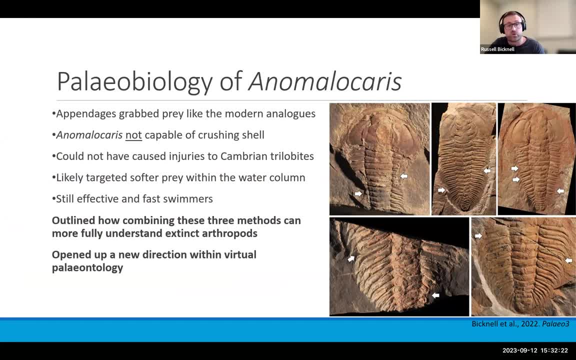 with these appendages, but it would have experienced a lot of stress or strain during that action, And so it probably was not, or most definitely was not, using these appendages to crush shelly things, So the array of trilobite injuries that we see in the Cambrian probably was not made. 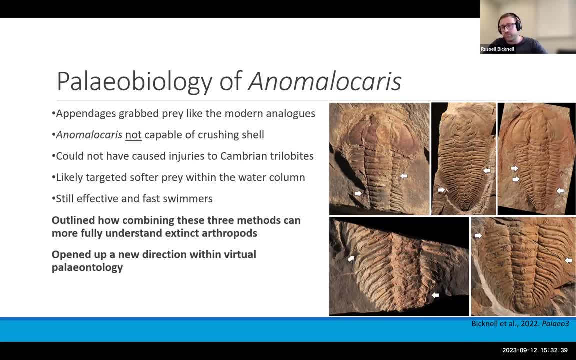 by Anomalocaris. It was more likely that this animal was swimming around in the water column and targeting the large diversity of soft prey that were also swimming around the water column, And so what we can say here by combining those three methods is: while this animal was not 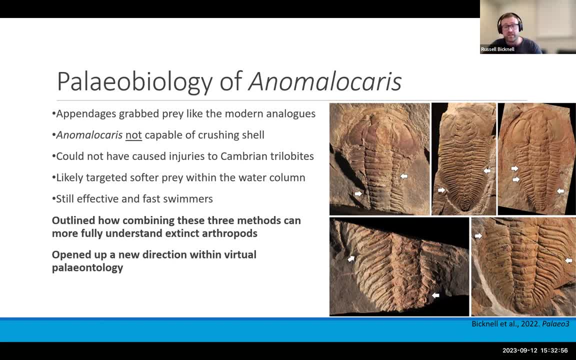 probably very good at actually tackling biomineralized prey. it was still a very effective predator, And so we can see that this animal was not very good at actually tackling biomineralized prey, And so we can see that this animal was not very good at actually tackling. 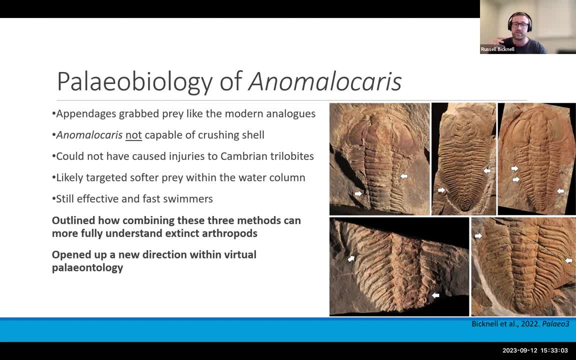 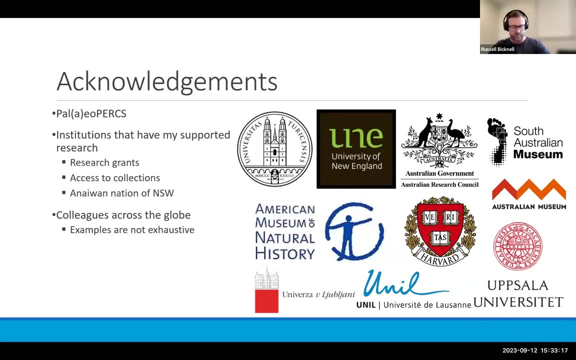 predator within the water column, And so really, this has allowed us to more fully understand and conceptualize how arthropods, in the context of predation, actually functioned in that bigger picture. Okay, well, that's the end of my talk. I think it's about 33-ish minutes Before I move on. 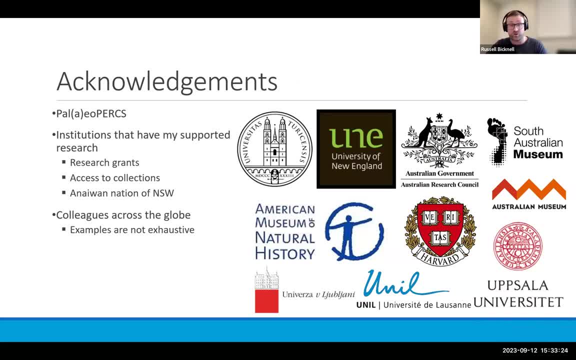 I just want to thank. there's an array of people I need to thank, because this work is not done by one person. This work is done by an array of brilliant academics, and so I just also want to say thank PaleoPerks for supporting this. This is such a great. 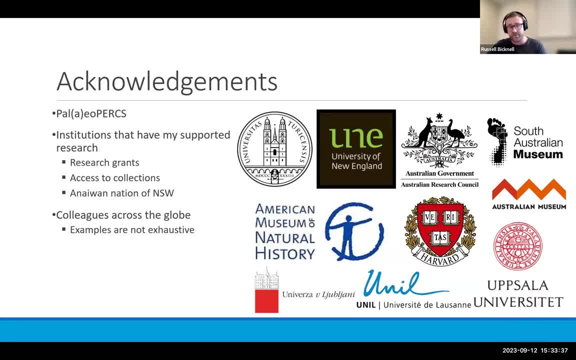 initiative and it's my honor and it's a pleasure to present to you today. There are so many institutions across the world that supported me either financially or in terms of access to material just being able to talk about this sort of stuff, And there are numerous more colleagues. 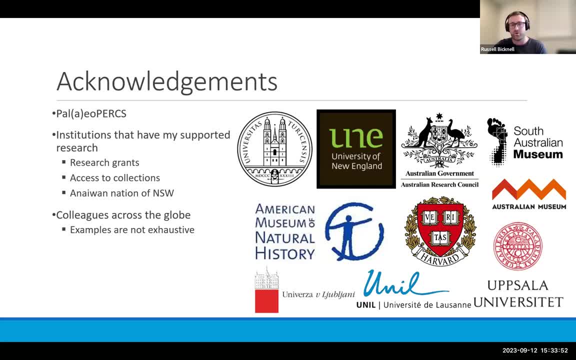 with whom I've had these sorts of discussions, of which I think at least there are two people here who I've co-authored my work with. So it's my pleasure to have worked and discussed these sorts of topics with these people. Thank you. 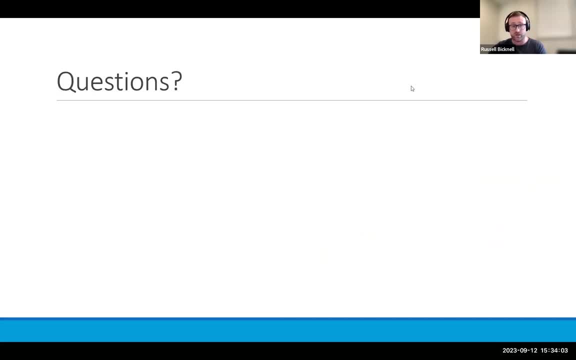 So thank you very much all yourselves for attending, and I think we now have time for questions. Yeah, great. Thank you so much, Russell, for that great talk and yeah, thank you everybody for joining us, and we do have questions that we already have. So I'm going to start by asking the 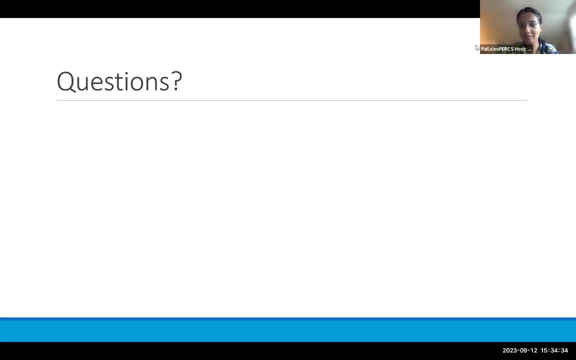 first one, and then I will also place it in the Zoom chat. The first question comes from Sender asks: how do you choose between either a phylogenetic analog and a functional analog while selecting a model organism for finite element analysis, For example? how would you? 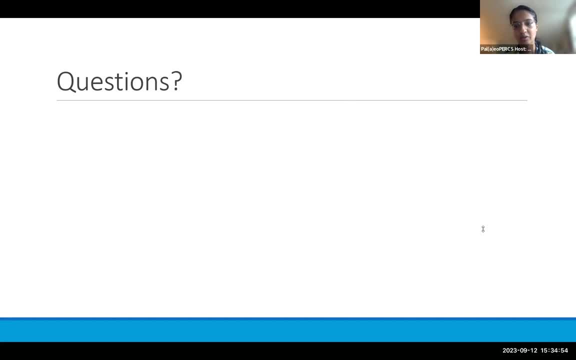 choose between a horseshoe crab and a normal anorine crab while preparing a FEA for eurypteride claws? Okay, this is a really good question. Partly sometimes you're limited by what we have in the day. So I had a very similar question when I was working on trilobites and horseshoe crabs is 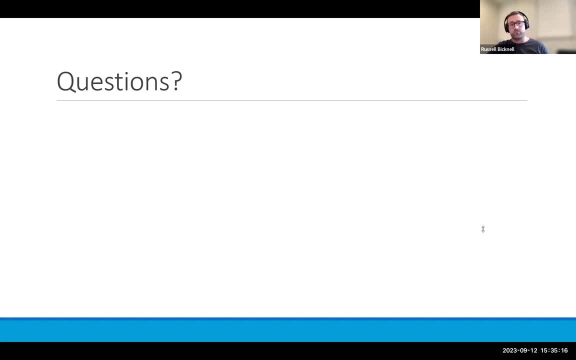 why didn't I use copepods? They also have nathabases. Well, copepods are a lot smaller than horseshoe crabs, So we're limited by the scope of what makes sense in that context. So in that, 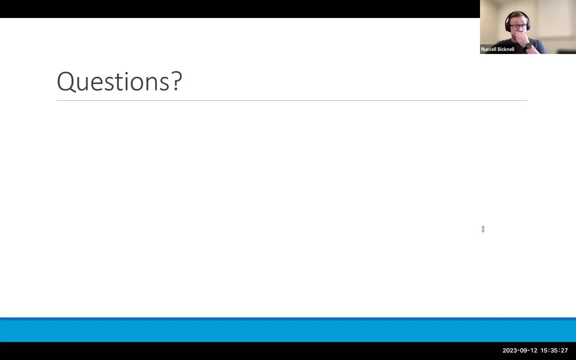 case it's functional morphology. In the case of looking at crabs versus chelicerates, that was a phylogenetic and functional morphological choice together. So we want to look at animals that are pretty close, Close to our fossil groups in terms of that phylogenetic bracketing. But also we can make 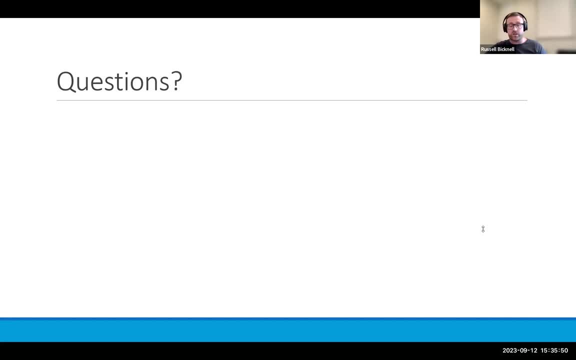 the assumption, given the way that we think that sea scorpions use the chelicerae, that it probably was closer to how scorpions use their pincers than how crabs use their structures. It also comes down to, I suppose, the way in which how the biology of the animals we're talking about. Finally, 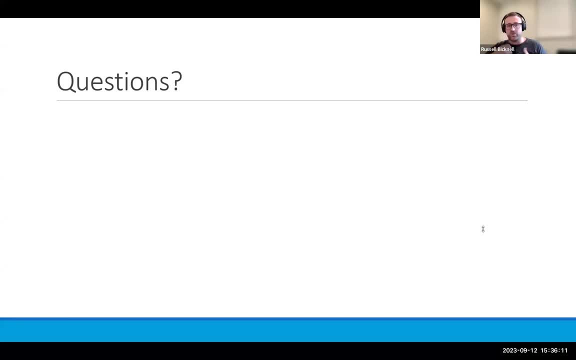 there's a material property aspect here that I didn't really go into because that's getting into the nitty gritty, But crabs have a very reinforced exoskeleton that we absolutely do not see in our sea scorpions, And so if we were to compare our crabs to our sea scorpions, 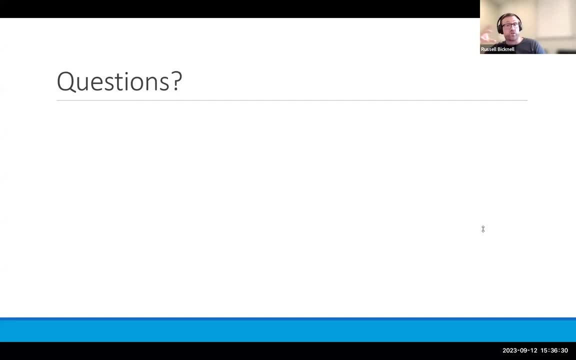 the models themselves for crabs would show a lot lower stress strain because they are more well reinforced, And so that comparison is then going to be really impacted by the that difference, which is going to influence how we interpret these models. Okay, great, Thank you. We have another anonymous question that has come up. 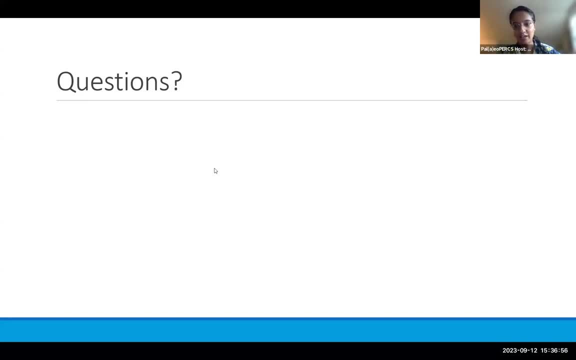 In your stress strain maps there were a lot of regions of high strain along specific parts of the chelicerae and other parts of appendages. Do you find that there is higher potential for breaking along those high stress points And is there any signal in? 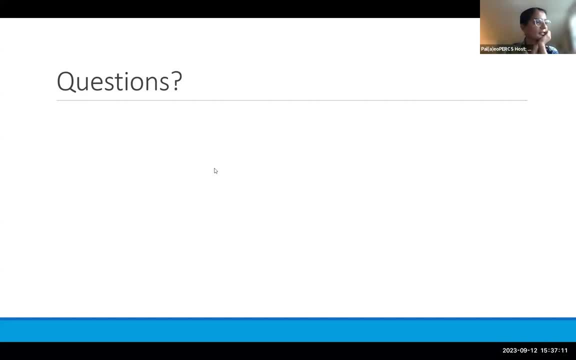 preservation that might indicate this. So we know that scorpions can. if you push a scorpion hard enough, like you can, it will experience failure in its pincer. But that being said, animals don't really tend to bite or pinch as hard as they possibly can. 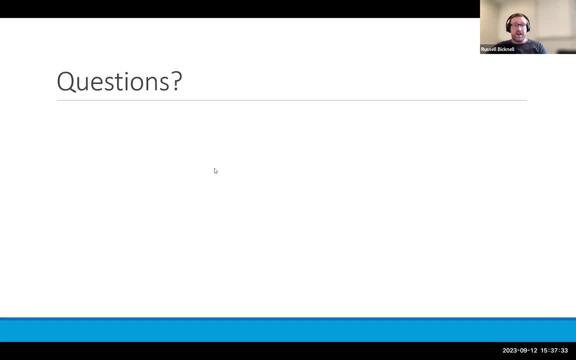 because that tends to result in some degree of pain and things don't like being in pain. So we can use our models to get an idea or where we may experience failure. but we are limited by the fact that these are models at the end of the day. so we can suggest, yeah, i mean maybe, um, it would experience this failure here. 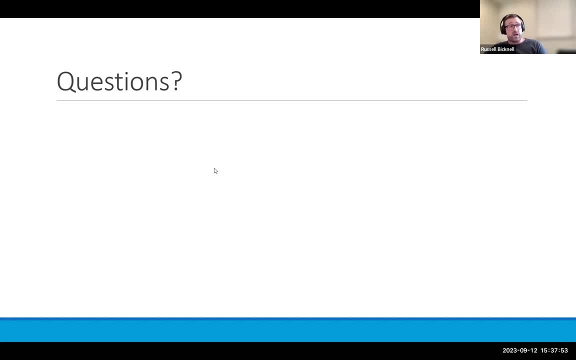 but we don't know for certain now. in the fossil record, to my knowledge, i have not seen any indication of these sorts of areas of failure, but also the majority of the animals that we looked at, at least from the sea scorpions- uh, there aren't that many chileus ray that have. 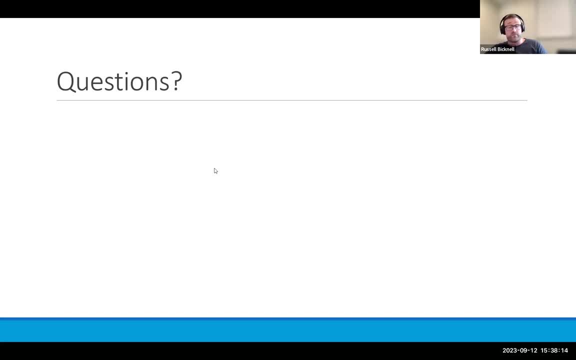 been preserved. so while they're really important technologically because of that requirement for soft body preservation, we don't see a ton of them in the fossil record which contrasts them like normal caris which we have like a lot of material from the burgess shale. so possibly is the answer. 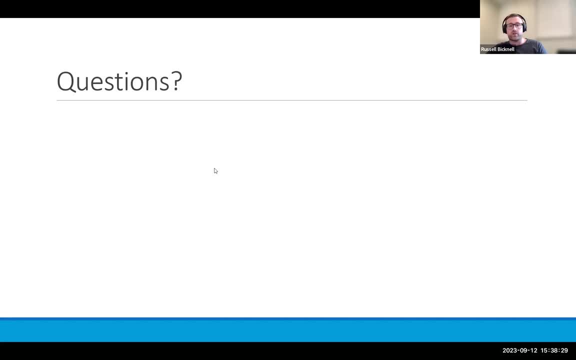 to that question, but there's not enough material for us to really kind of determine that and ground truth that idea. great, thank you for answering. we have another question by sender that i've also dropped in the zoom chat: have you tried plotting the fea data with? 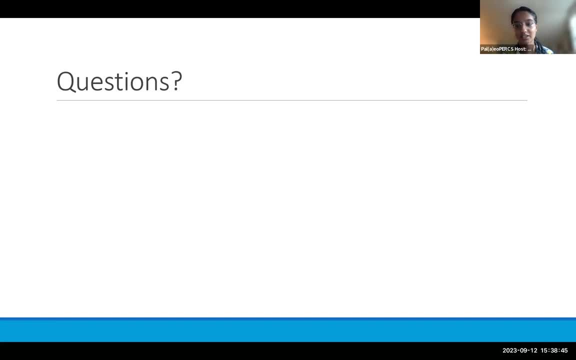 a morpho space concerning the group on which the fe is conducted, in this case with the tyrol gotids, and a step further: would incorporating the phylo morpho space be of importance and help answer questions relating to the ecological position a group occupies? yes is the answer. 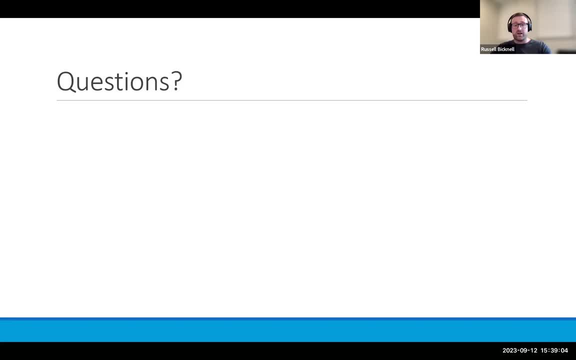 to that question, and that is effectively the current frontier of my work. um in terms of accessibility, so done it for scorpions, um, and the limitation there is that the scorpion phylogeny needs to be rebuilt. um, so i can't necessarily build a complete phylo morpho space, but i can at least. 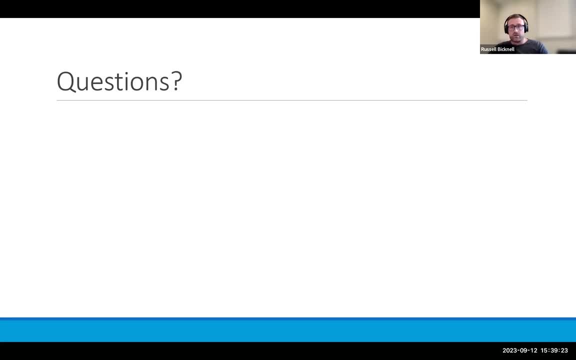 look at where these animals are, i suppose, constructed or where they fall, when we look at the the geometric morphometrics of the shape of these structures. and so it does show you is that there are definitely places in the morpho space where certain scorpion pencil morphologies do tend to cluster. 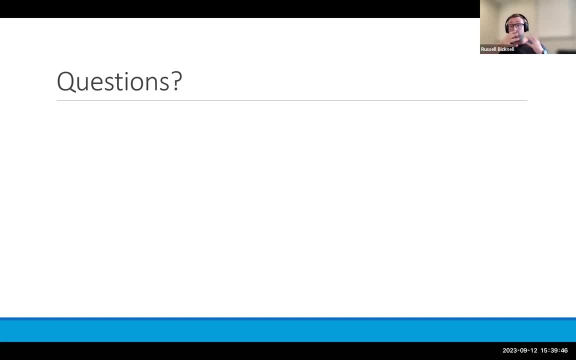 and this gives you an idea of really what that yeah, the ecology of these sorts of animals as well, and this kind of builds on work that's also being done to understand the eco morphotypes of scorpions in general. uh, and longer term, i'd like to look at this, uh, in crabs and also sea scorpions. 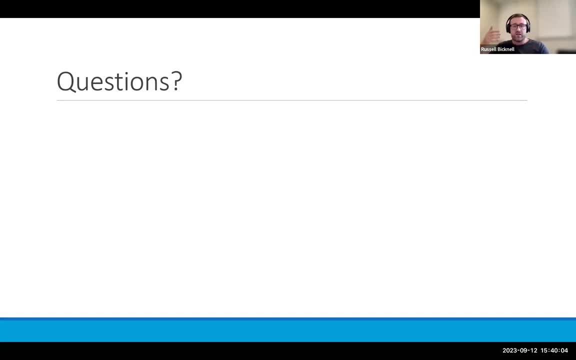 and any other kind of pincery, like things we see in the fossil record today. to really understand like: why do pincers keep evolving over and over again? there must be something in the utility of these structures and i think we can really explore that by building these sorts of phytomorphic spaces. 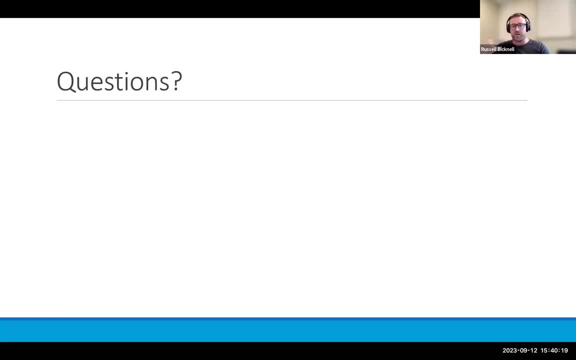 the answer is yes, um, and we just watch the space for the next three years while i build the tile models, and we'll see. great, yeah, there's, there's a sort of trailer for what's coming up next. right, exactly, yeah, um, so we have a few more questions, um, and again, if people want to ask, 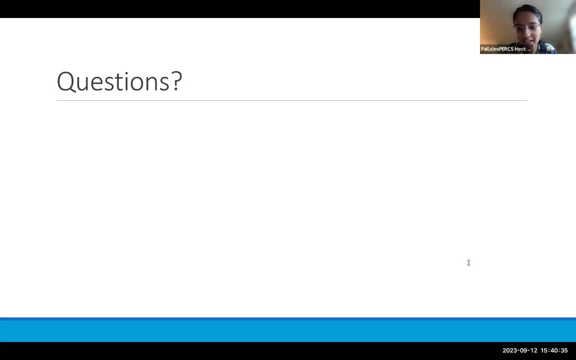 questions directly in the zoom chat, um, or you can also raise your hand, please feel. feel free to do so, um. we have an anonymous question and the question is: does the computational fluid dynamics model allow for changes in the sediment flow that is not just a fluid, but closer to different brackish? 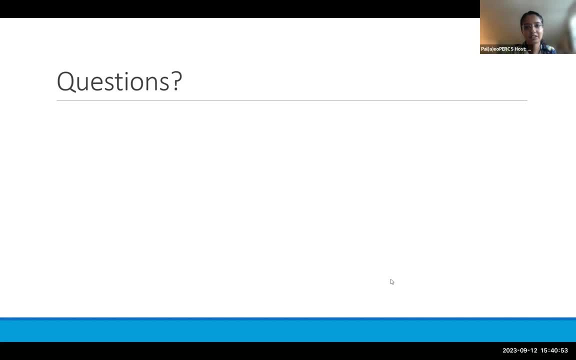 conditions which had sediment flow. yes, um, we can specify the density of water, that's all the density of the fluid. so you can use cfd to like understand how birds fly. obviously, birds don't fly through water, they fly through the air, and so you can adjust your fluid to be density of air, and so, yes, you can increase the density. 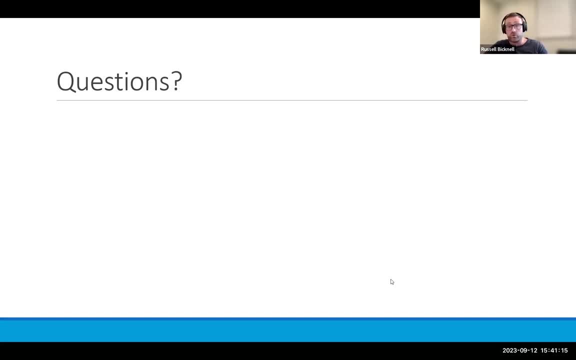 of water, based on what you think a brackish environment would be, and that absolutely would be part of that consideration, although the the flip side of that is, when you start to build in those additional aspects to your model, your model becomes harder to compare with other things. so 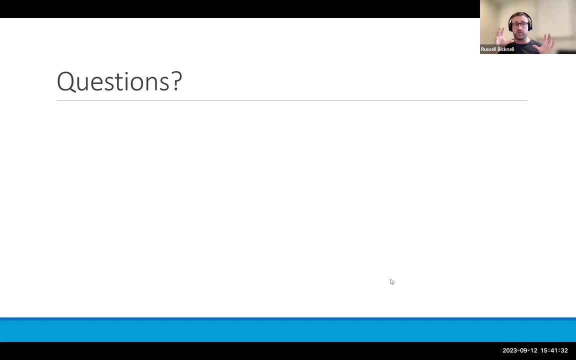 really, whether or not you want to include that level of information is really a case by case thing, in the same way that i didn't look at crabs to understand pincers because the material properties would be markedly different. whether or not we want to start to look, 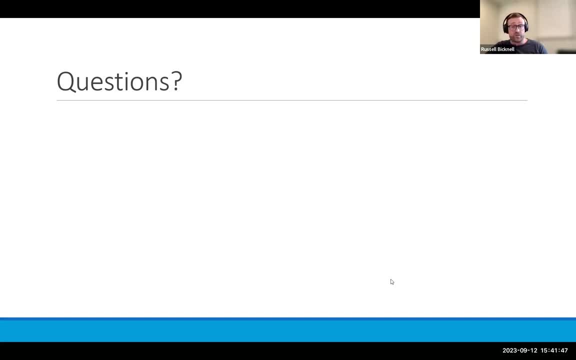 and include that level of density in our computational fluid dynamic models does come down to the question we're trying to address. great, uh, we have a question by shannon um that i'm dropping again in the chat is: do you think that, in addition to attacking soft-bodied prey, some of the animals in questions might still go for hard-shelled prey, if the prey? 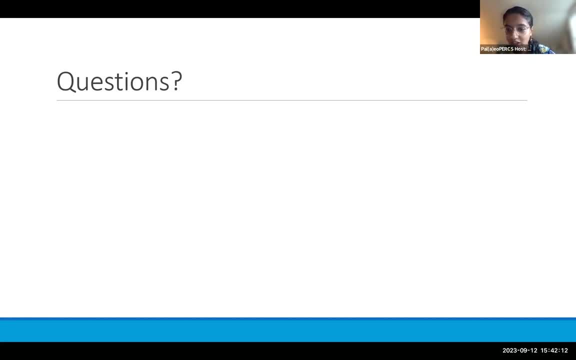 was already injured or if they'd scavenge dying ones? on a related note, can models consider the effects of struggling prey versus grabbing a motionless object, which maybe can be analogous to targeting weaker individuals or scavenging um? so to the first part: yes, we know that. when arthropods molt, they give off some kind of chemical which is thought to be able to attract predators. and so yeah, during a post-malt stage and during that sort of redevelopment of the exoskeleton, it's very possible that these sorts of animals would have been attacking. 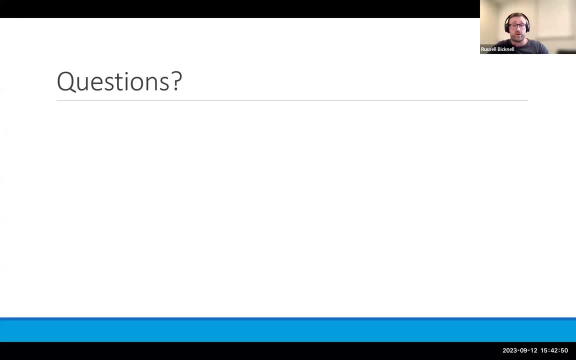 uh weakly by mineralized prey items. on the topic of modeling, struggling prey kind of um. so this has been done. for crocodiles, people have looked at uh different angles of attack and have looked at different, i suppose, uh conditions for biting the hard part with this sort of animal. 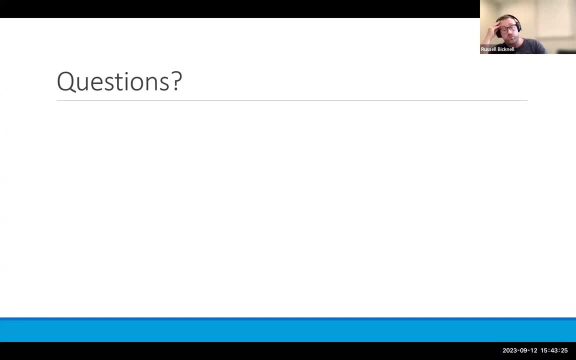 is we. if you think about normal chorus, we don't really know what the articulation with the, the head of the animal, really looks like. so we already have a lot of assumptions built into this, but we don't know what the articulation with the, the head of the animal, really looks like. 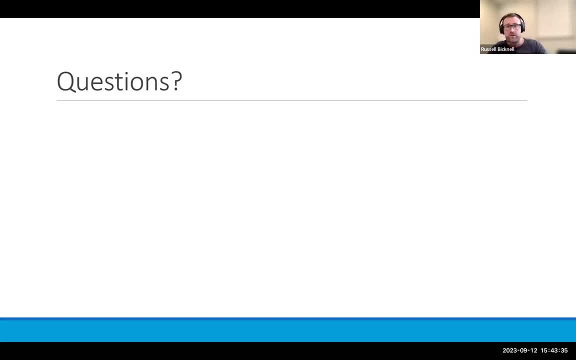 into our model. but to have that kind of additional aspect, you would need to have that additional part of the body which introduces an additional array of assumptions and also introduce the question of how did this appendage move in the head socket, which we, we don't know, uh, arthropods like. trilobites are a lot easier. the appendages are in in an array, so like modern day horseshoe crabs, and so we can make the assumption that they probably weren't able to necessarily twist prey so much and it would have been a lesser problem in that context. so yes, it's possible. 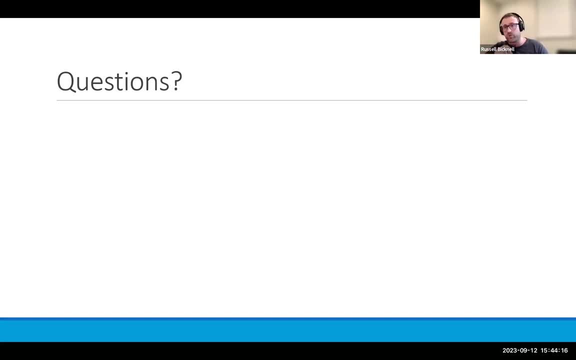 whether or not it's plausible is is a different question, and whether or not it's sort of worth, the number of assumptions that you know immediately skyrocket, and we're already talking about a lot of assumptions here. uh, that's, you know. really, you reach this point of 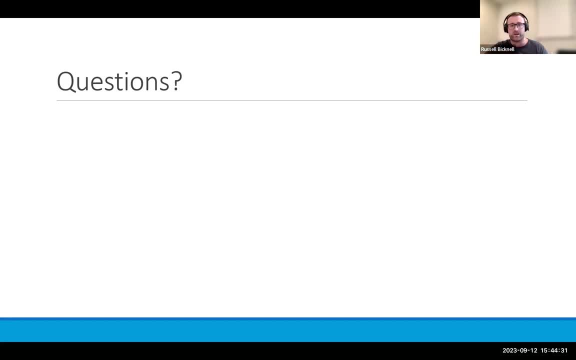 at what point are we? you know, almost making something up just for a cooler story, and i'd prefer to err on the side of caution with these sorts of models that already are full assumptions. great, thank you for answering the question. we have one more um. okay, i think i copied it twice, so i'm going to copy it more times so it just doesn't just um. 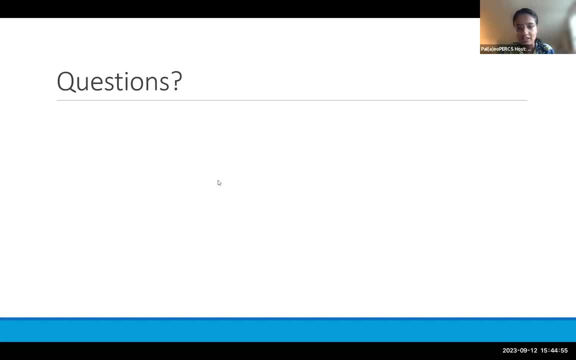 okay, so this question is again by sender and the question is so he says this question is little more on the speculative side. how would you design a FEA study for some of the Vendor-Bion's idiocarin taxons which lack to a major degree any modern analogs? I wouldn't to be entirely candid. 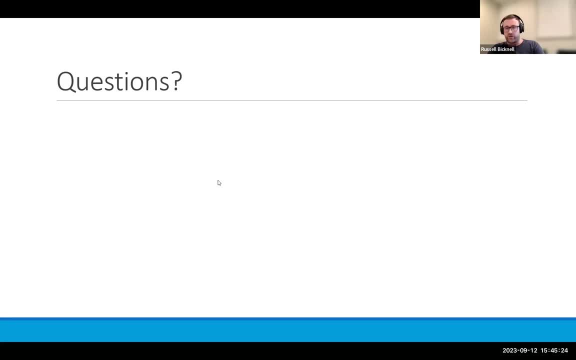 FEA is one of those interesting tools where, once you start using it, you can almost get into the point of like you know, everything looks like a hammer, a nail if you have a hammer, and you can use it to understand more and more animals. but for me, I've sort of come to this place of being. 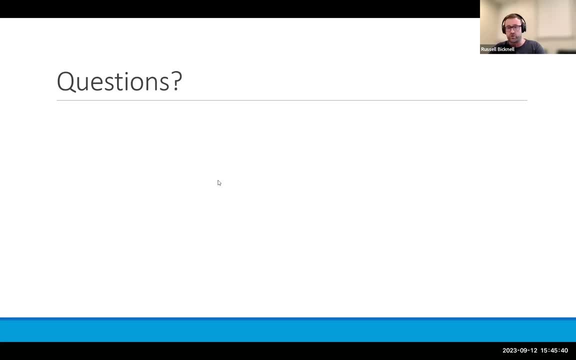 of really asking like: is that method actually appropriate for whatever I'm trying to do With idiocarin things I mean? so many assumptions work, their sound, like computational fluid dynamics of these animals, like the method section is so long for like one paragraph of results and so 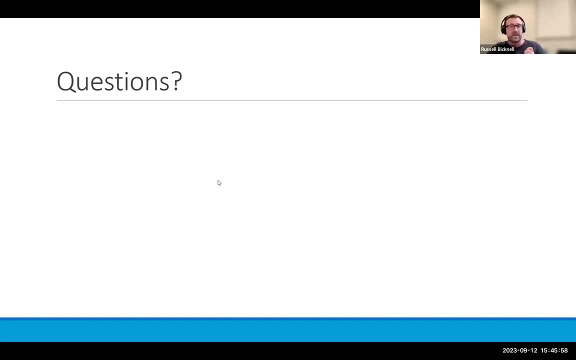 I wouldn't even really want to try and step into that realm in that context, But I think beyond that, the kinds of methods that are more appropriate. there are methods like computational fluid dynamics. they're methods like three-dimensional geometric morphometrics, because they are more within the realm of like understanding how the environment. 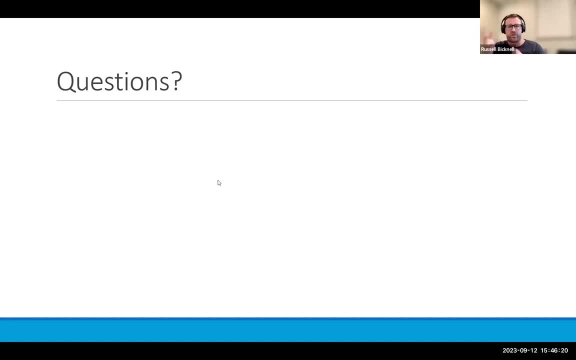 is impacting the animal, as opposed to what the animal is doing on other things. Great, thank you for fielding all the questions and if anybody has more questions, we can take those over to Tim. And once again, thank you, Russell, for giving a fabulous talk. I will take over screen share. 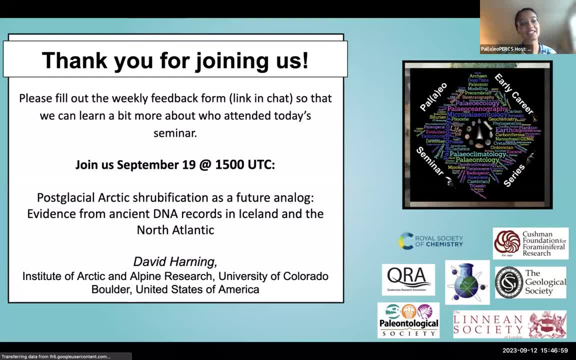 Okay, thank you everybody for joining us Again. you will find the link in the chat for the weekly feedback form. In addition, you'll also find the link for nominating early career researchers. Join us next week where we will have David Harning from the University of California. 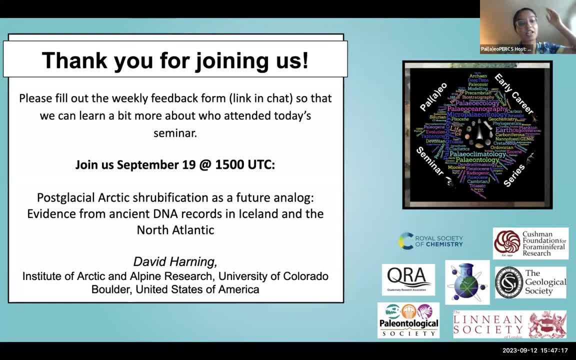 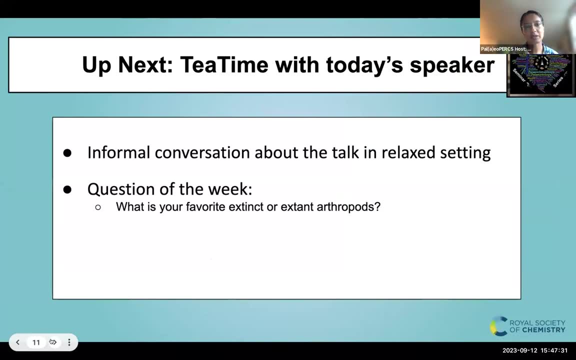 Colorado, Boulder, and he will be talking about post-glacial arctic shrubification as a future analog evidence from ancient DNA records in Iceland and the North Atlantic. Up next is tea time with today's speaker Russell is graciously taking time out to spend it with us, So it will be an 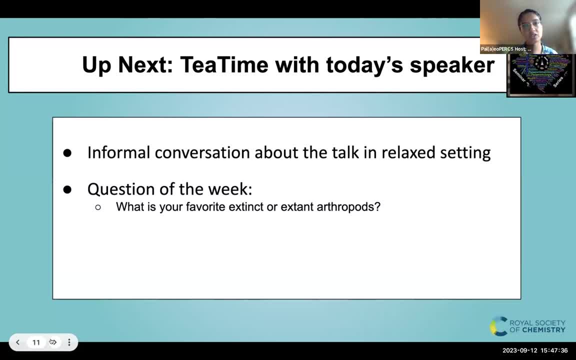 informal conversation about the talk, as well as any other questions about academic trajectories that you would like to ask. To kick things off, the question for the week is: what is your favorite extinct or endangered species, And if you have any questions, feel free to ask them in the Q&A box. 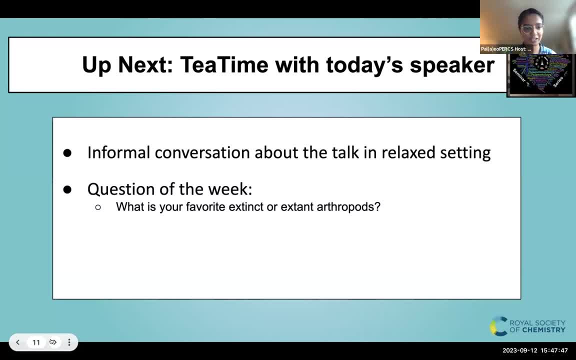 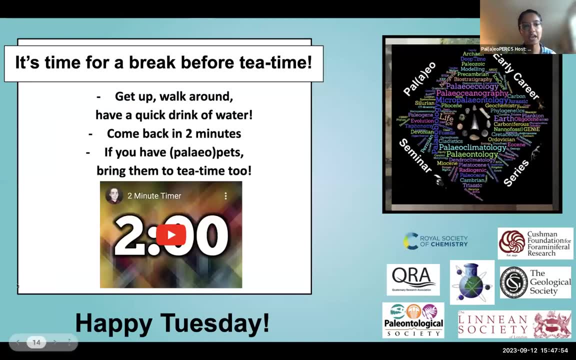 Thank you so much for joining us today. We will have a two-minute break, so this is your time to get up, walk around, have a quick drink of water, and we will all reconvene in two minutes. Thank you.